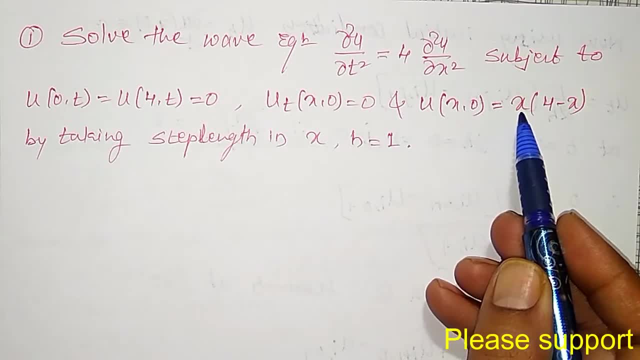 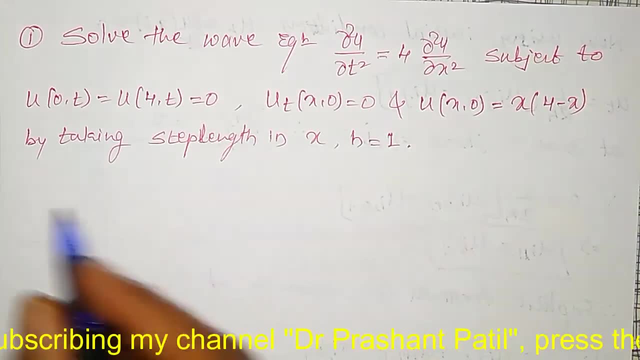 and u of x comma 0 equal to x times 4 minus 0. That is 4 minus x by taking the step length in x, as h is equal to 1.. First of all, let me compare this one with the standard form of wave equation. 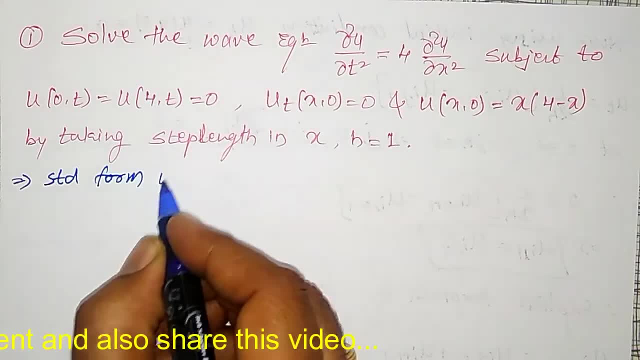 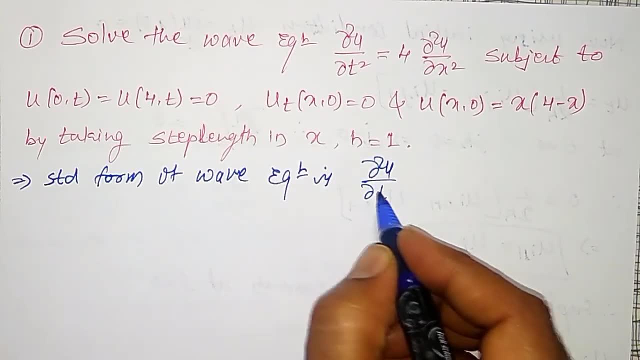 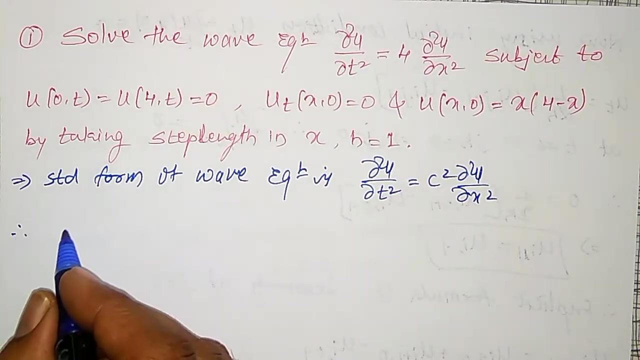 Standard form of wave equation is: dou square u by dou t square, equal to c square into dou square u by dou x square. Therefore my c square value is equal to 4 here. If c square equal to 4, then c is equal to plus or minus 2.. 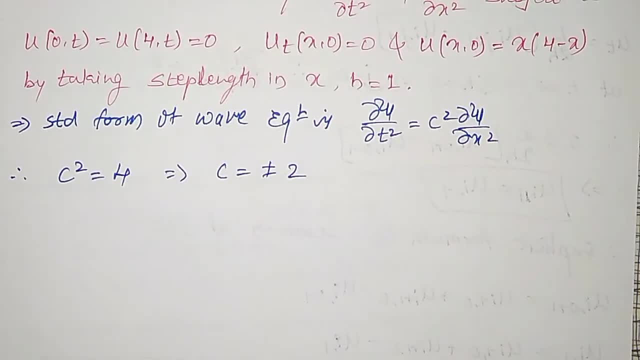 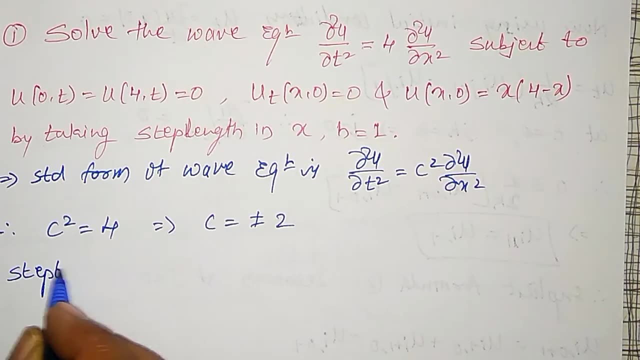 But I am taking only plus 2 here- Then by comparing the step length, they have given Step length in x, as h is equal to 1.. Therefore, step length in t k must be equal to h divided by c. To apply that explicit formula. 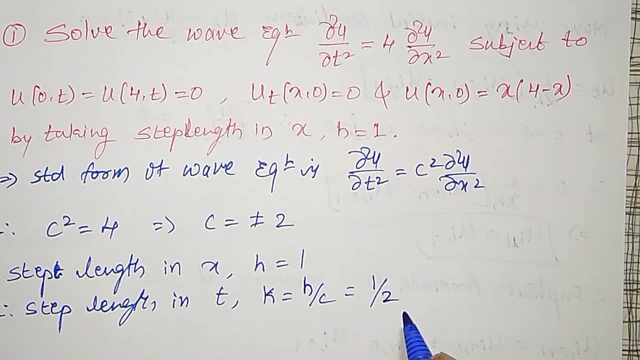 Where h value is 1 and c value is 2.. Therefore, I can use: it is equal to 0.5.. h is equal to 1, k is equal to 0.5. I have to use Then. what is the equation? 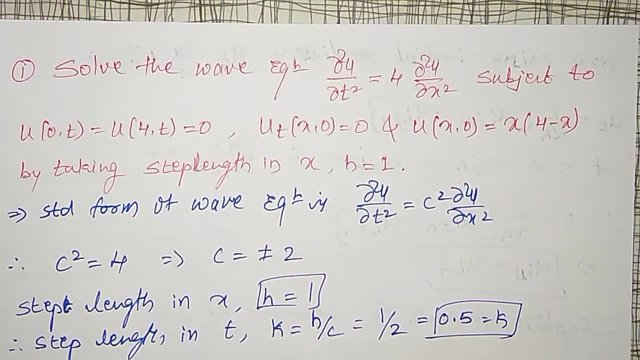 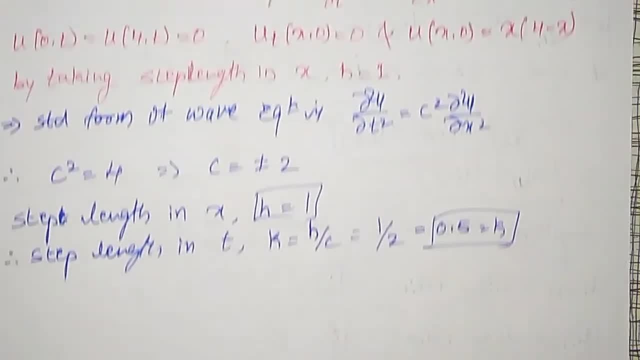 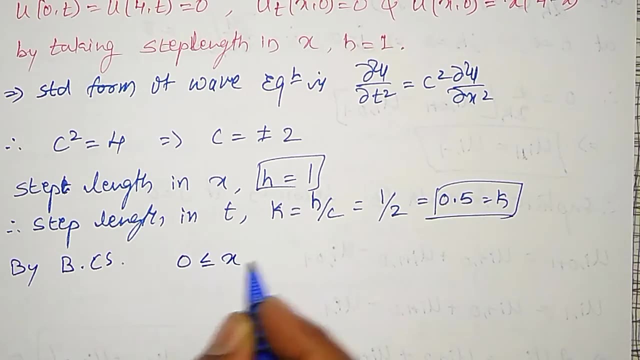 Here one thing. you can just check What are my boundary conditions: u of 0 comma t equal to u of 4 comma t. Therefore x is varying from 0 to 4 here By the boundary conditions. 0 is less than or equal to x, less than or equal to 4.. 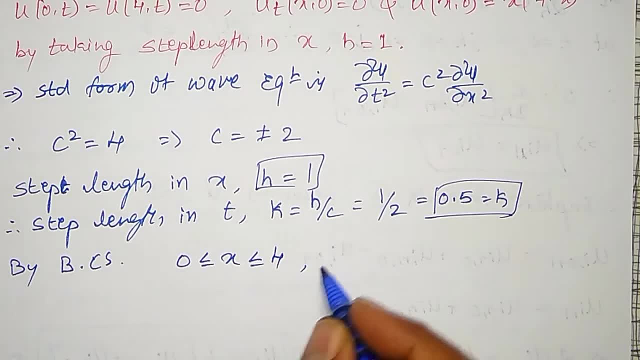 x is varying from 0 to 4.. Which is divided by Which is divided as, Divided as x0 equal to first 0. Then x1 is equal to x0 plus h. My x0 value is 0.. h value is 1.. 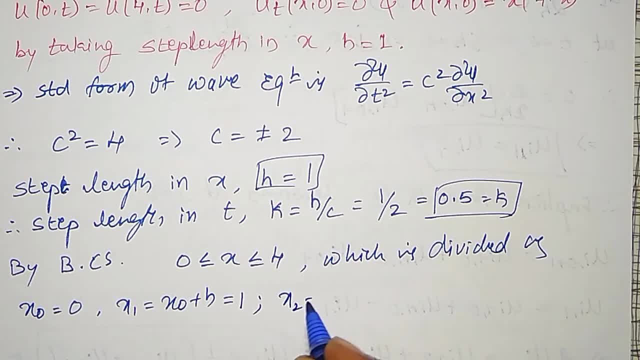 Therefore equal to 1.. Next, x2 equal to x0 plus 2h, x0 is 0.. 2 times h. 2 into h is 2.. And x3 equal to x0 plus 3h. 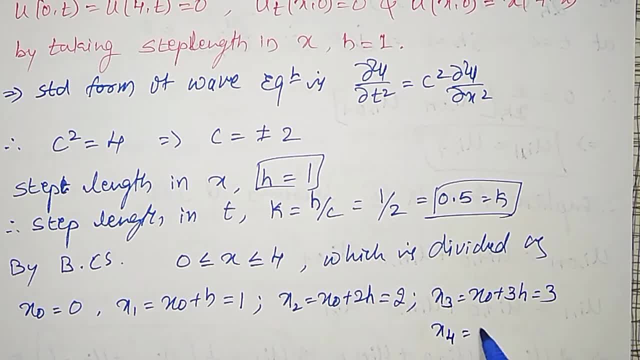 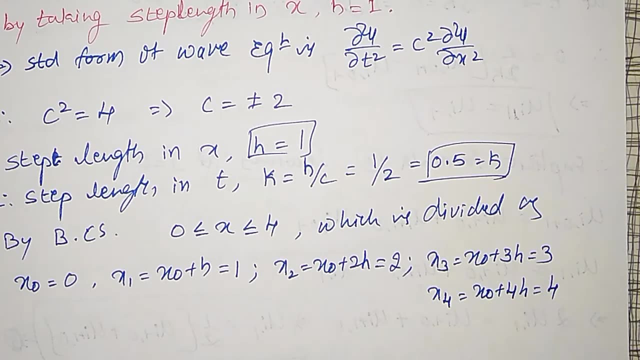 That is equal to 3.. And x4 equal to x0 plus 4h, Which is equal to 4.. Therefore, 0,, 1,, 2,, 3,, 4 are divided into parts Like that. my t also. I will divide equal up to t4 only. 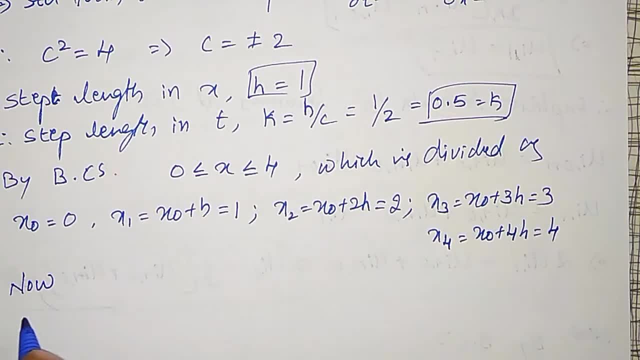 Now t0, initially t value, that is, the time- is 0. Then t1 is equal to t0 plus k. k value is 0.5.. Therefore I am getting 0.5.. 0 plus 0.5.. 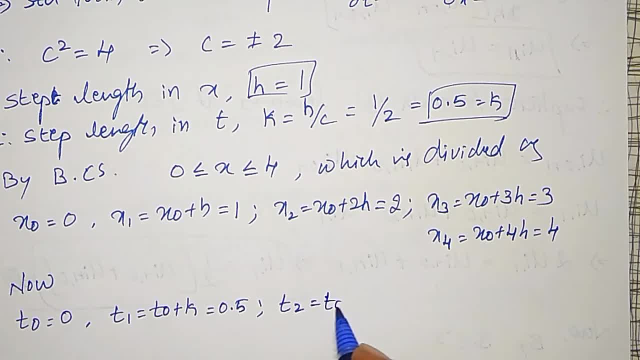 Next, t2 equal to t0 plus 2k. 2 into 0.5 is 1.. Like that, t3 equal to t0 plus 3k, t0 is 0.. And 3k will become 1.5.. 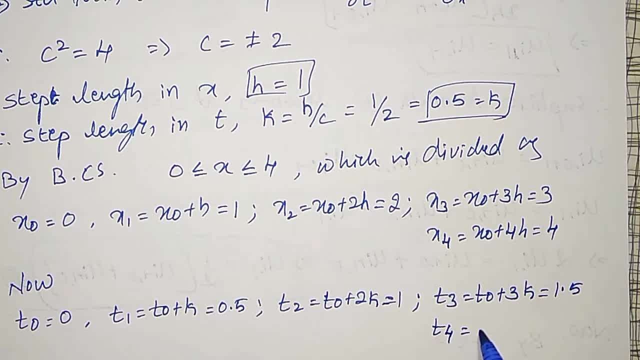 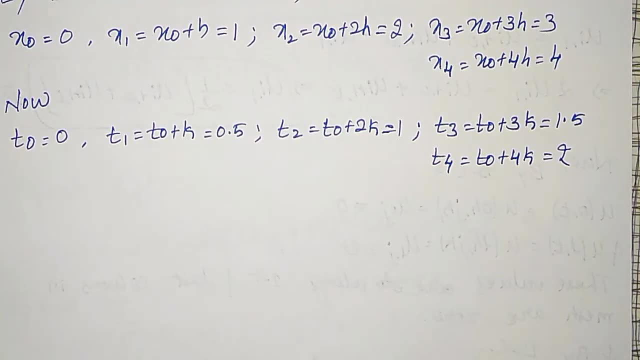 Like that: t4 is equal to t0 plus 4k, 4k raised to 2.. Okay, Therefore, x also, y also. I have divided Using them. using these values of x and y values, I will form the table. 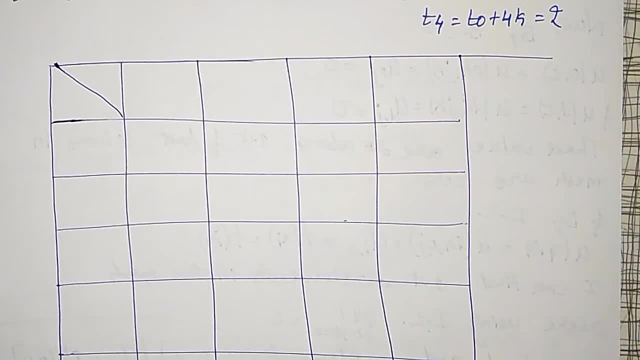 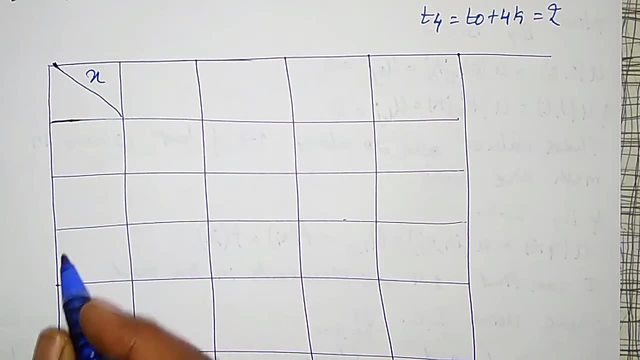 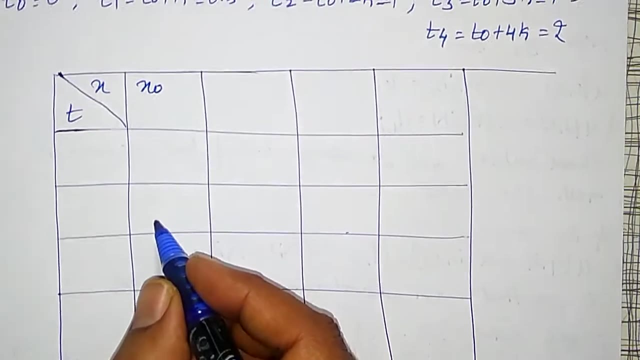 And I will come back here as, while forming the mesh, along columns, I will take it as x values And along row value, I will take it as t values. Therefore, this is my x0.. Okay, And x0 value from the table. you can just check here. 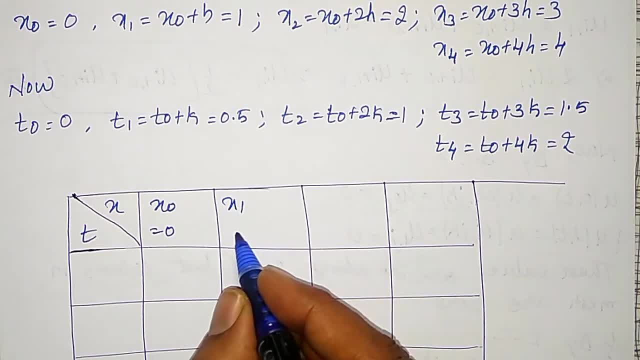 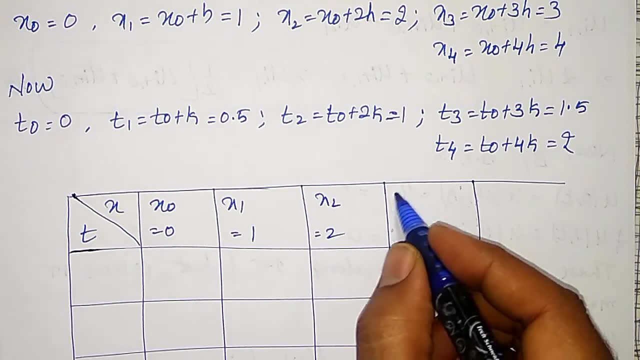 It is equal to 0.. x1 as second row, that is equal to 1.. x2 equal to 2.. x3 equal to 3.. And x4 equal to 4.. I am going to use here Like that, along the first column, t values. I will take. 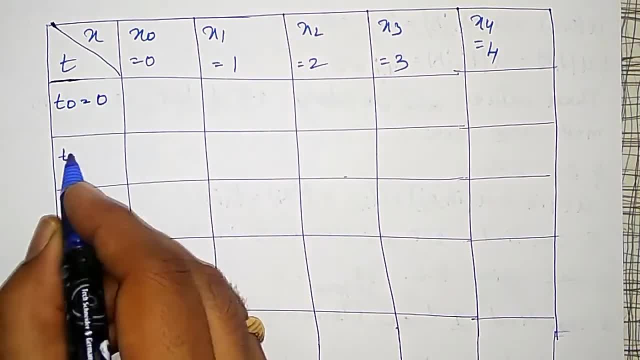 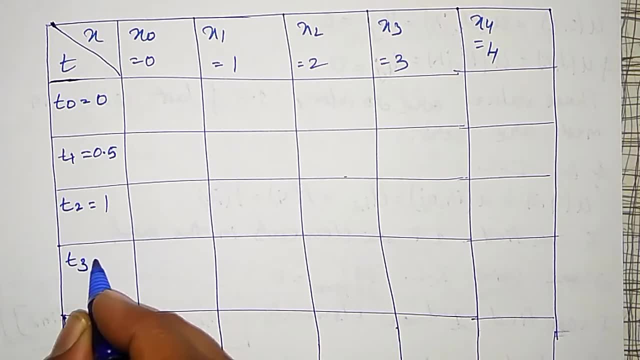 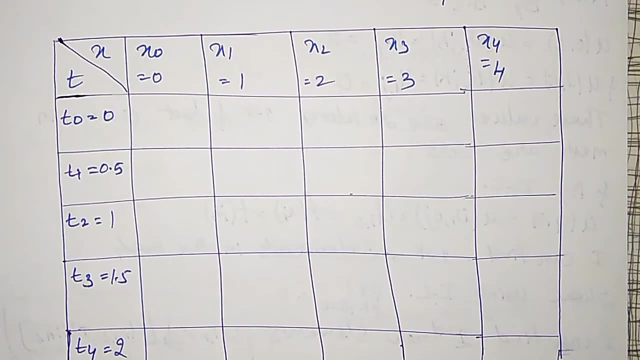 That is t0 equal to 0.. t1 equal to 0.5.. t2 equal to 1.. t3 equal to 1.5.. And t4 equal to 2.. Now using these values. first this one. 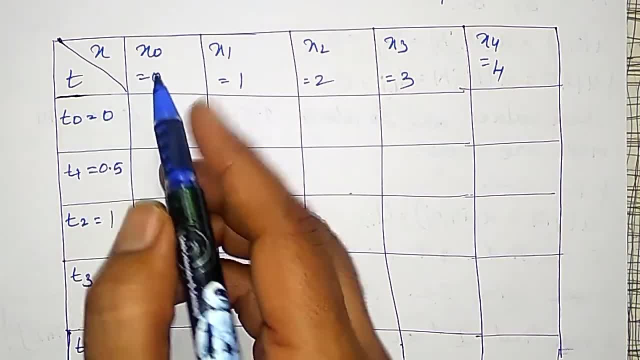 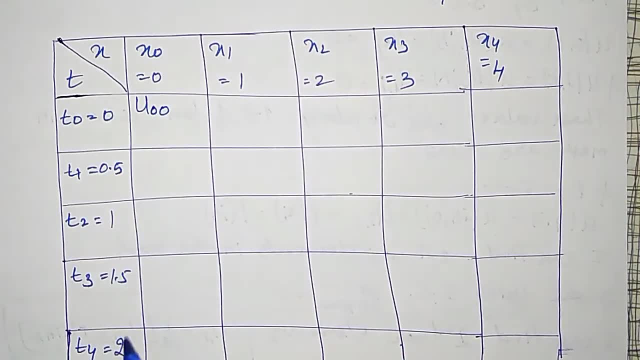 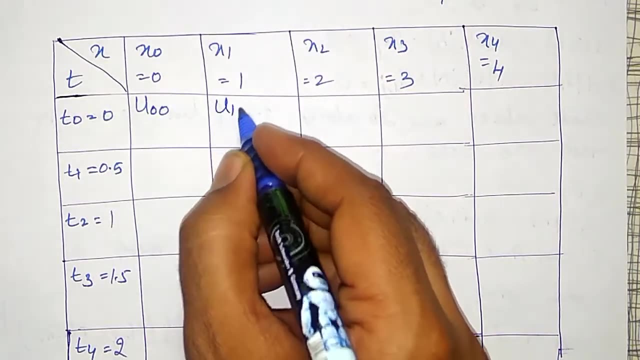 the suffixes I am going to use to notation them. Therefore, first one will become u, That is u u. Therefore, its notation is u. This one is u. This is u, This is 2.. And this suffix 2 I am using. 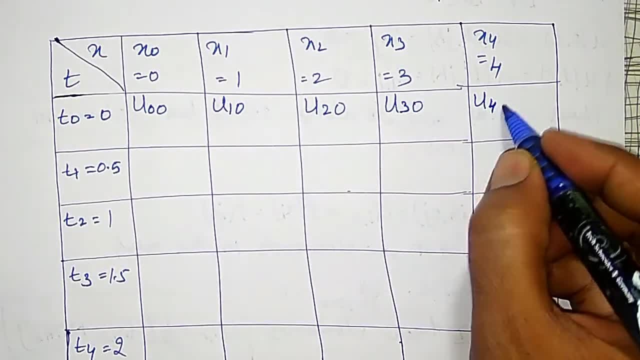 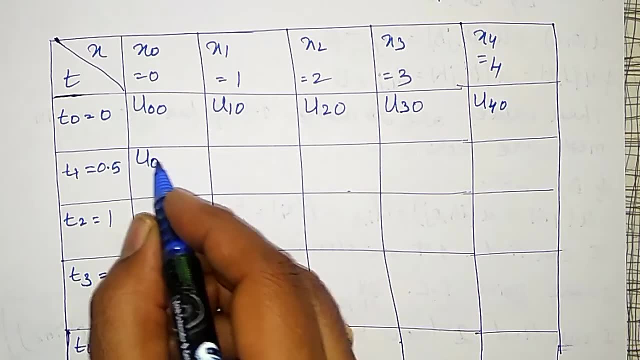 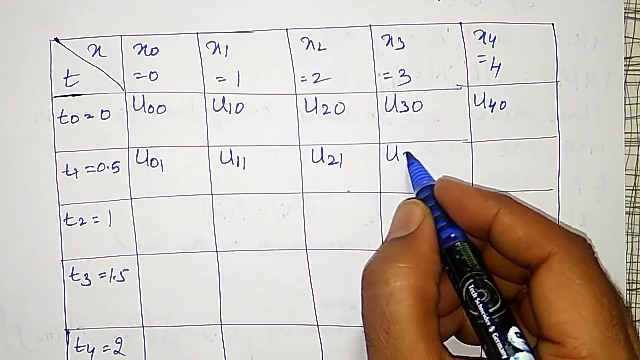 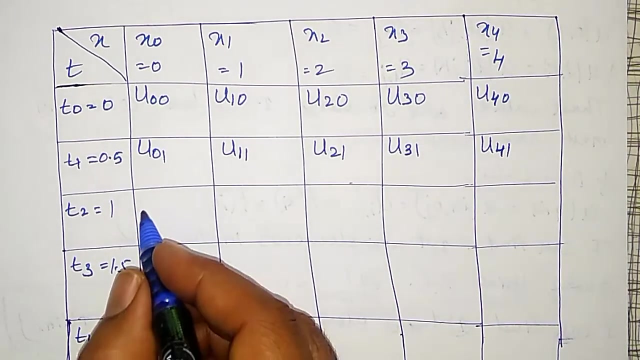 u And this notation is u I am going to use. Like that, second row will become u u u u u. Like that, I will write the remaining also. That is u and then t, That is 0,, 2.. 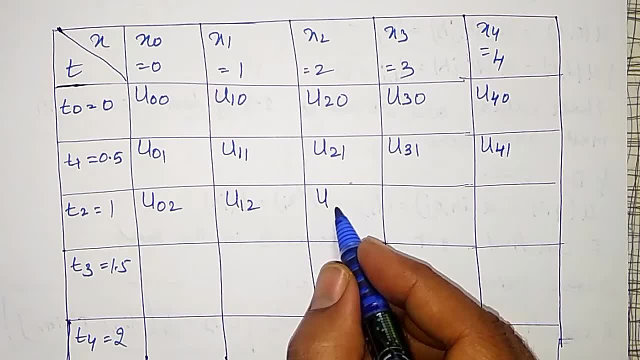 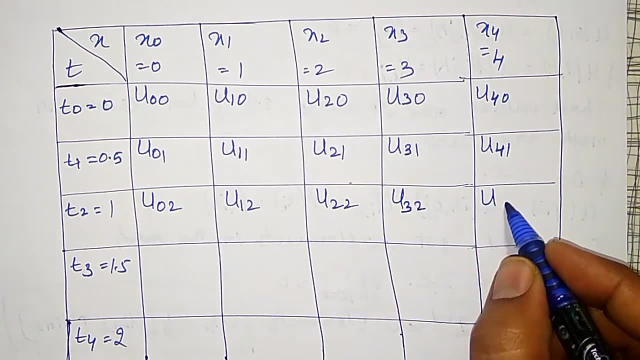 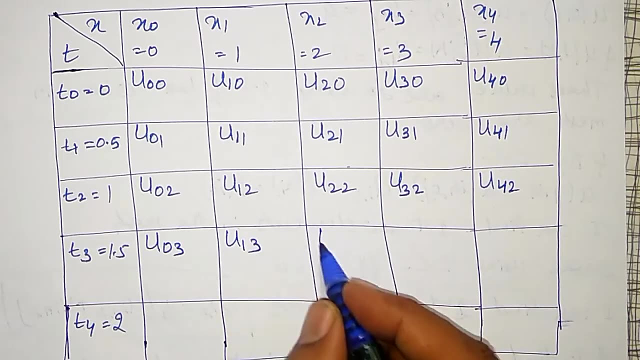 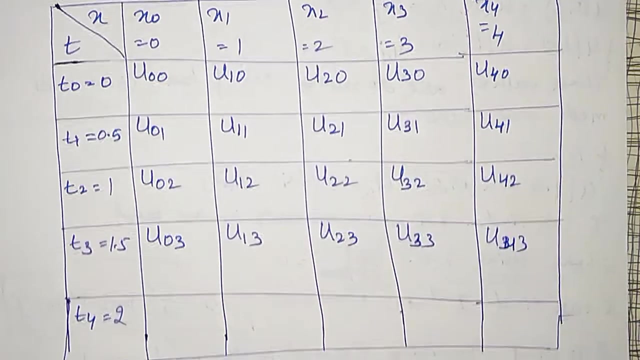 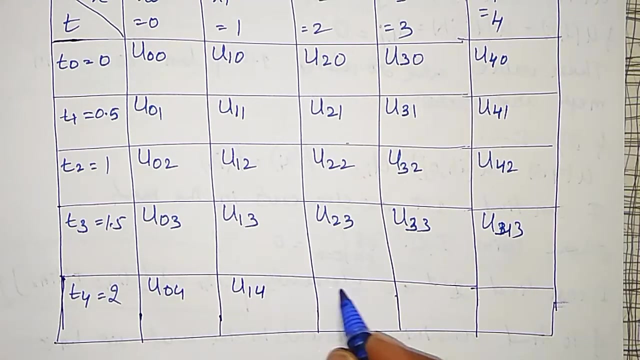 u u u u u u 0, 3, U of 1, 3, U of 2, 3, U of 3, 3, U of 4, 3, like that last one: U of 0, 4, U of 1, 4, U of 2, 4, U of 3, 4, U of 4, 4. 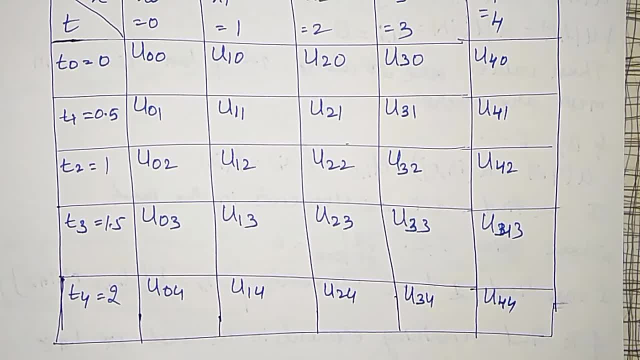 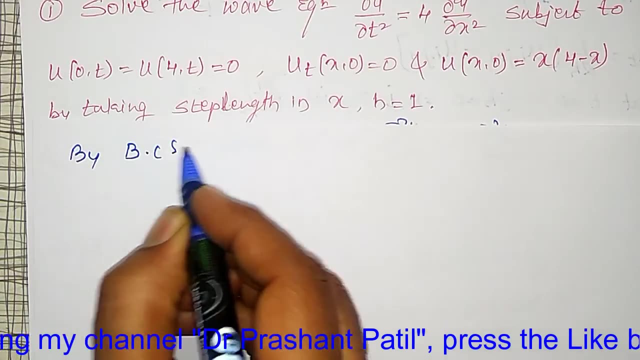 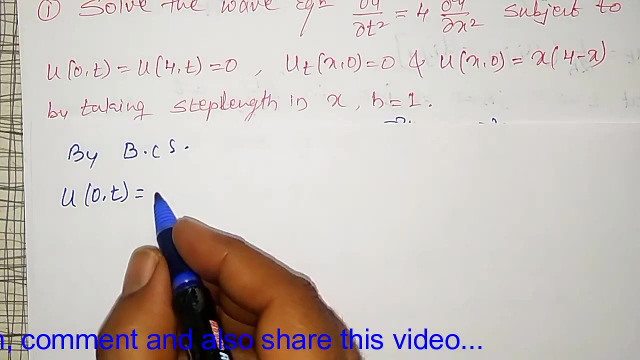 these values I have to calculate one by one. to calculate them, I am going to use the initial conditions first, one by one. I will come back here now. let me use the boundary conditions. by boundary conditions, U of 0, t, that notation is nothing but 0, x equal to 0. 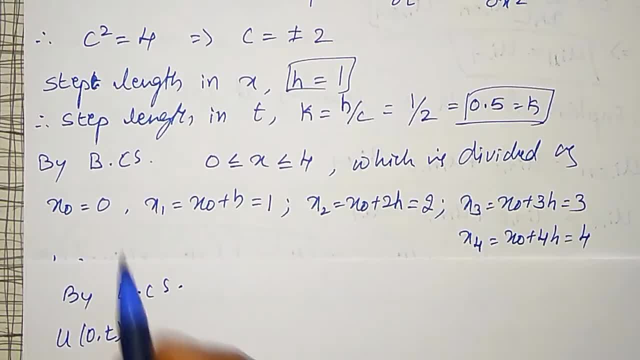 is for x equal to 0, is for x0 equal to 0. therefore I can write it as U of x0, comma tj. I can write correct: that is equal to U of 0, j, j values taking different values. but x value is 0, which is equal to 0. 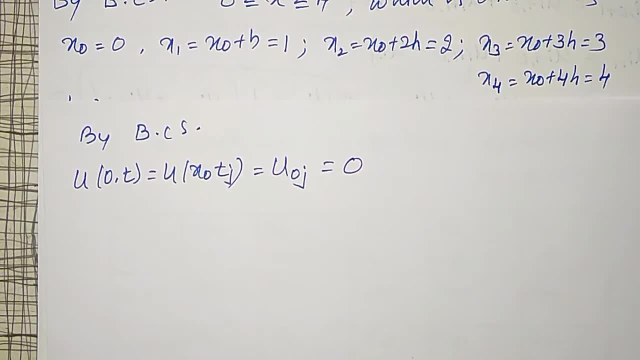 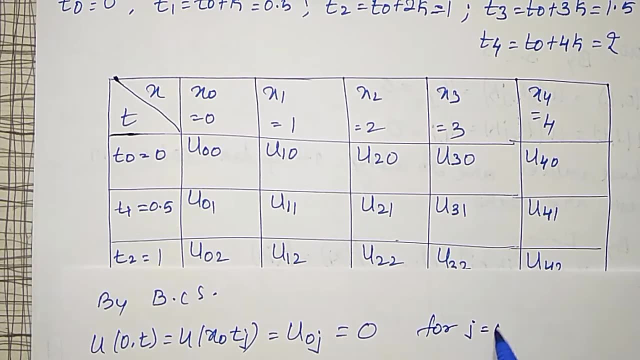 therefore, in your table U of 0, j, 0 first is 0, rest all j is taking for j equal to 0, 1, 2, 3 and 4. all these values are 0. therefore, my first column values are 0. using the condition U of 0 t x0. 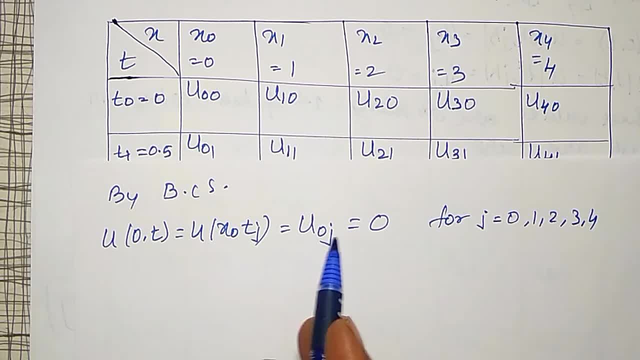 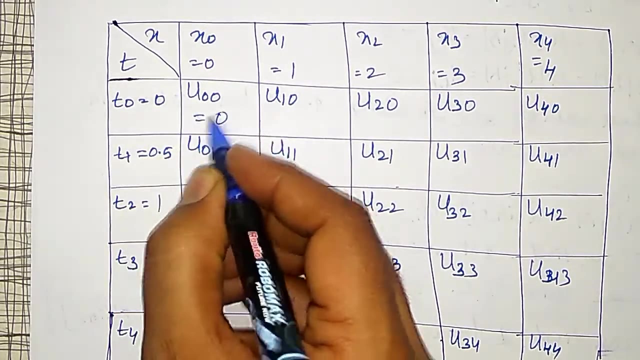 0 is for x0, tj, therefore 0, j. that is equal to 0. that is first column. are 0 elements correct? I will write in the table also first column: this is equal to 0. this is equal to 0. this is also equal to 0. 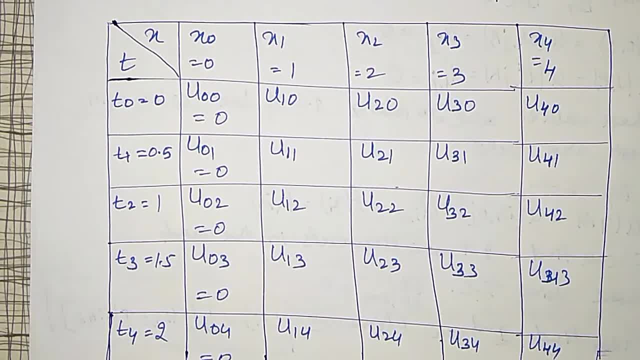 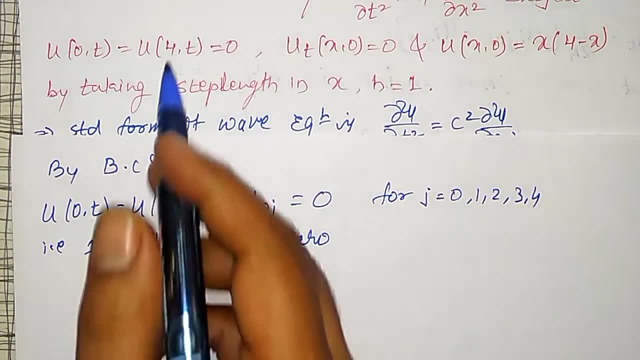 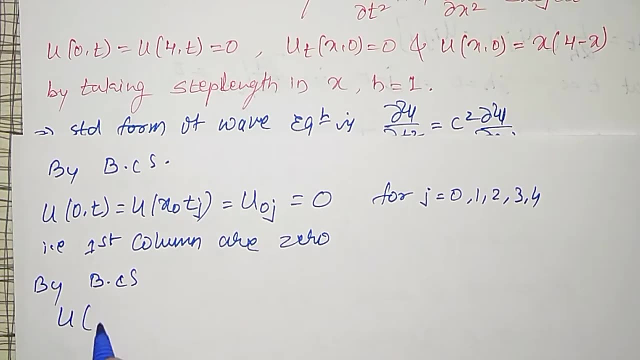 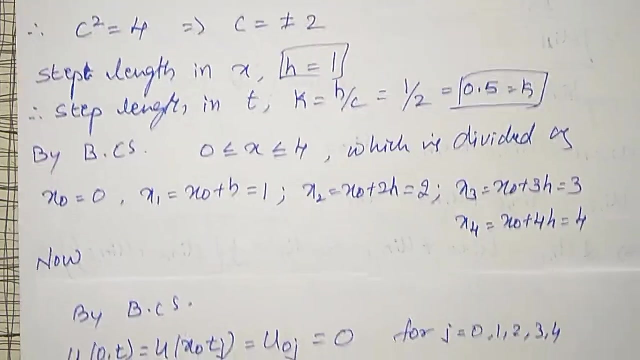 this is equal to 0 and this is also equal to 0. ok, like that, using another boundary condition. what is my another boundary condition here from that given for problem by boundary condition? U of 4 comma, t equal to and x equal to 4 is for. 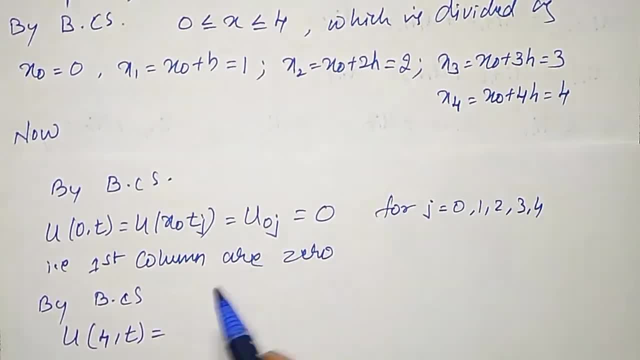 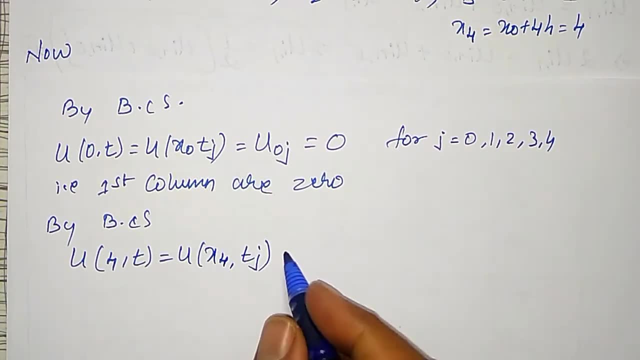 according to what I divided, x4 equal to 4. therefore this one I can write it as U of x4, comma tj. I can write- that is short notation- U of 4, j equal to 0. for again j equal to 0, 1, 2, 3 and 4. 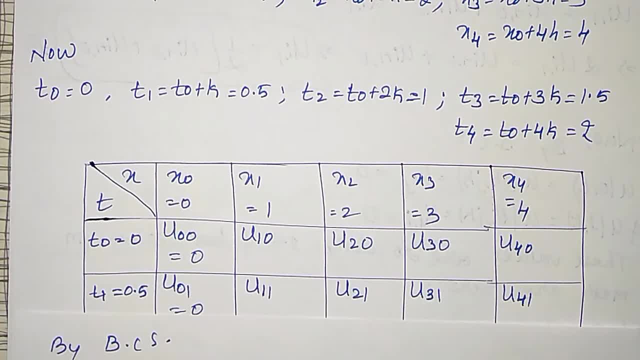 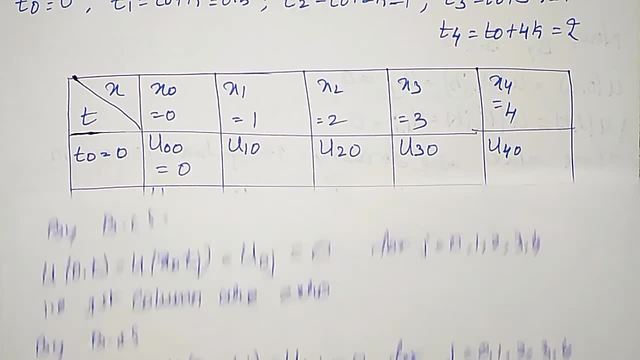 what it shows then. U of 4 comma j, that is U of 4 comma j, last column. U of 4: 0, 4, 1, 4, 2, 4, 3, 4, 4. all these values are also 0. that is last column. 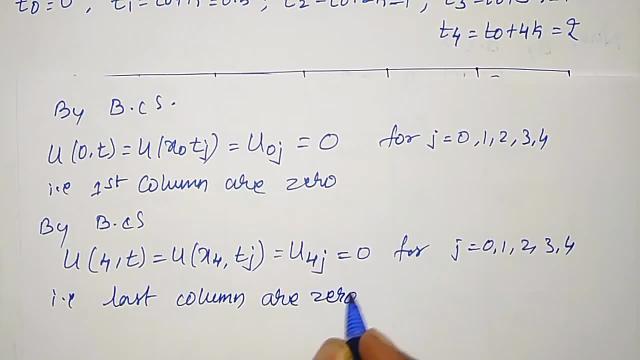 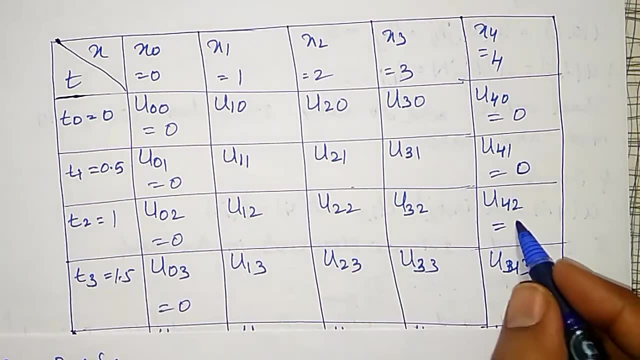 column are 0 here. correct. therefore: U of 4- 0 equal to 0, U of 4- 1 equal to 0, U of 4- 2 equal to 0. in the table, U of 4- 3 equal to 0 and U of 4- 4 also equal to 0. 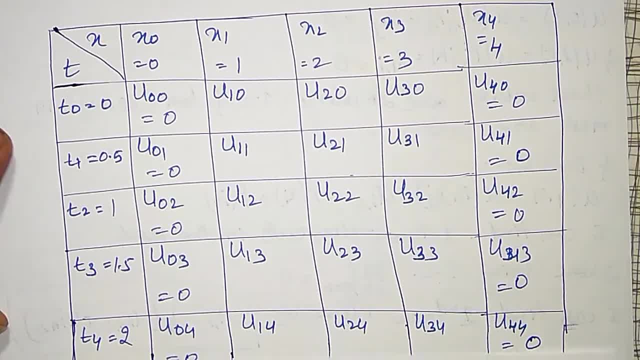 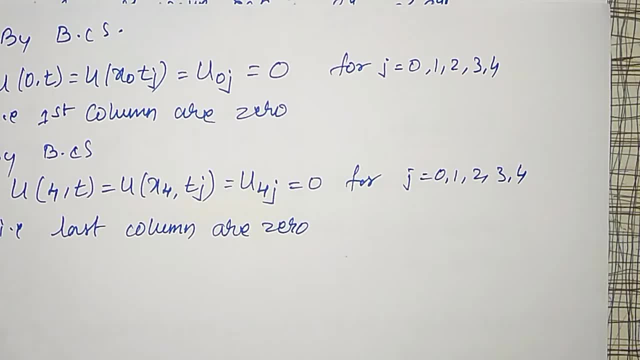 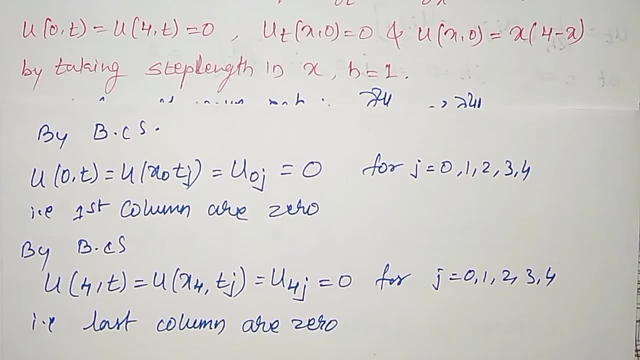 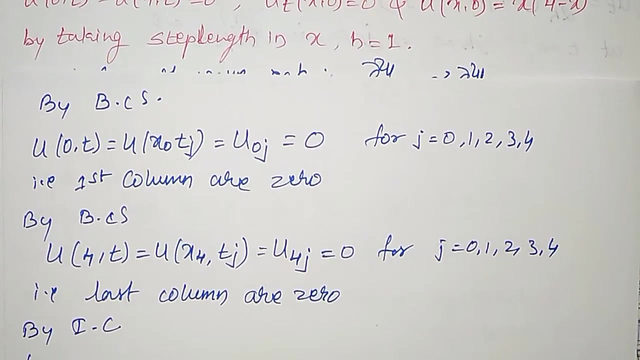 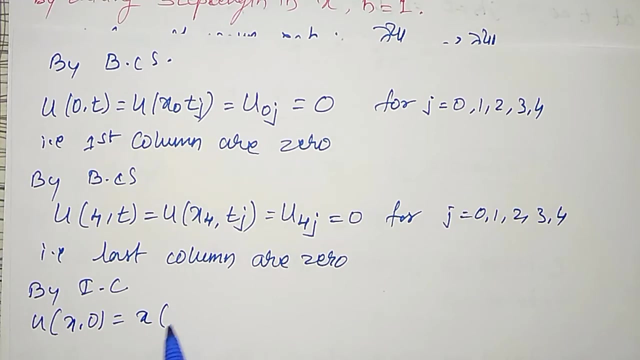 from the table. ok, this is using two conditions and next, using initial condition. what is my initial condition? next one, my initial condition is: next now using the initial condition. last initial condition I will use by initial condition U of U of x, comma 0, equal to x times 4 minus x. 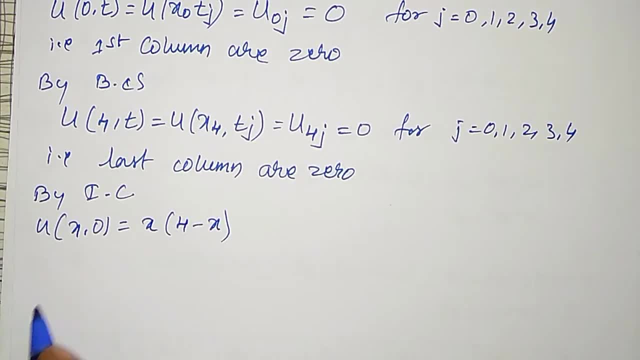 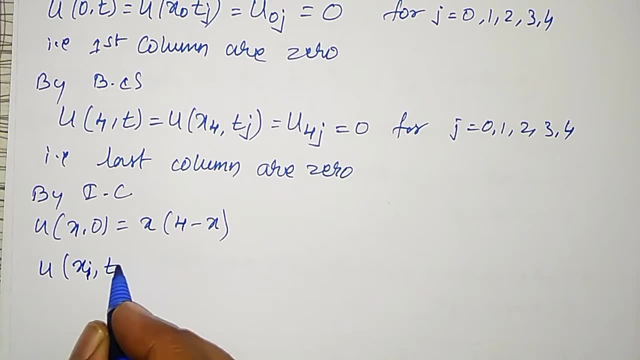 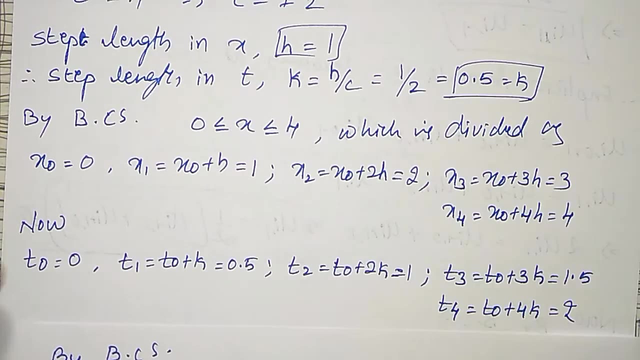 ok, my short notation for this one is that U of U of x i comma correct x i comma t naught, that is, U of t naught is t naught is equal to sorry. 0. t naught is equal to 0. 0 for t naught. 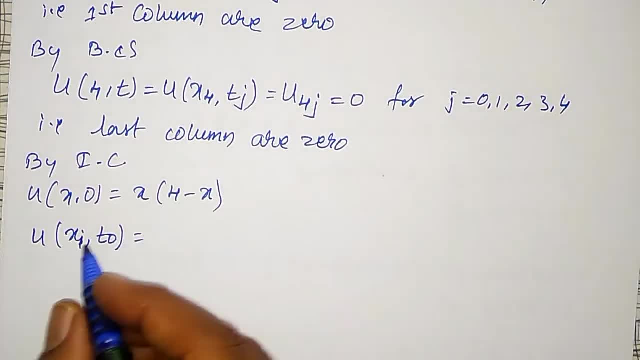 that is why t naught I am using here, therefore. therefore, this is nothing but U of U of i comma 0, U of i comma 0. that is x i into 4 minus x i for i equal to 0, 1, 2, 3, 4. 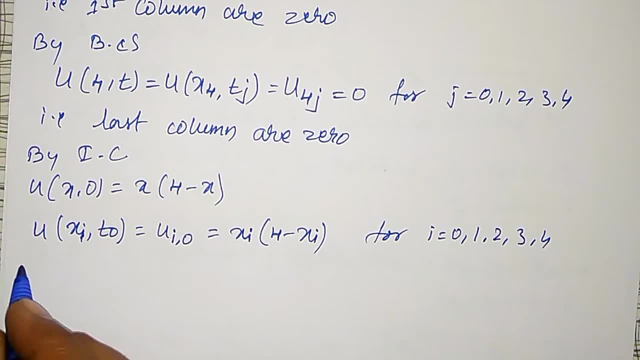 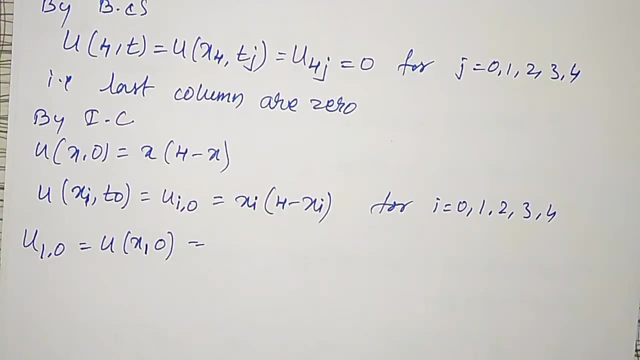 ok, now let me substitute one by one. therefore, U of 1 comma 0 equal to U of x 1 comma 0. what is my x 1 value from the divided? what I divided, x 1 is equal to 1. using that x 1 into: 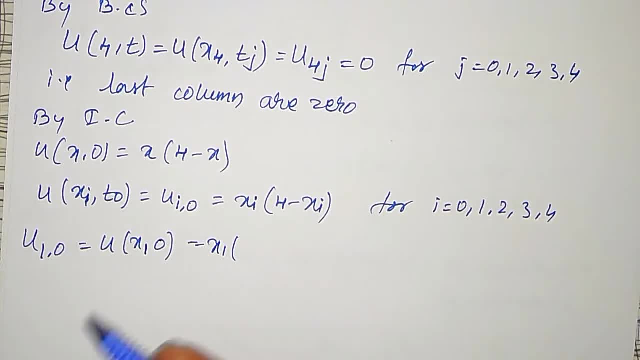 sorry, before that 0, 0 you can find out i equal to 0. for confusion, let me find out x naught first: x naught into 4 minus x naught. but x naught value is 0, 0 into 4 minus 0, equal to 0. 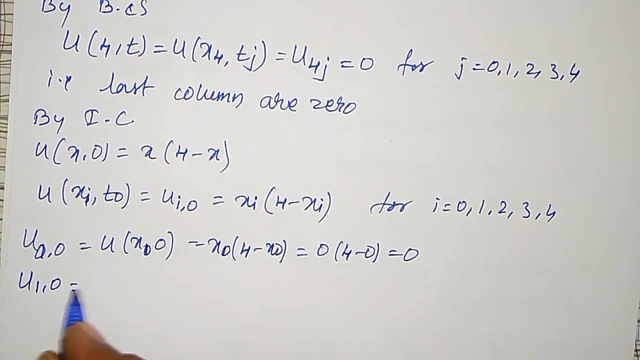 like that: U 1 comma 0, U 1 0, that is U of x 1 comma 0 x 1. value x 1 value x 1 into 4 minus x 1, but my x 1 value is 0. x 1 value is 1. 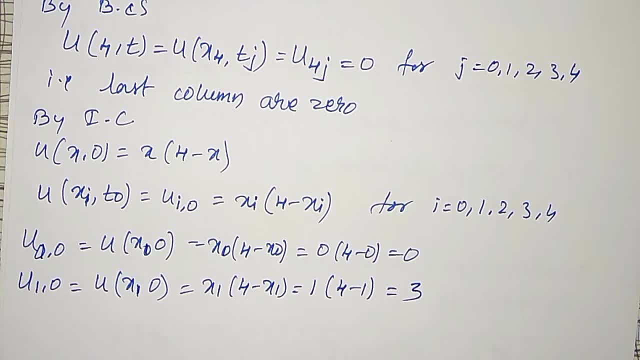 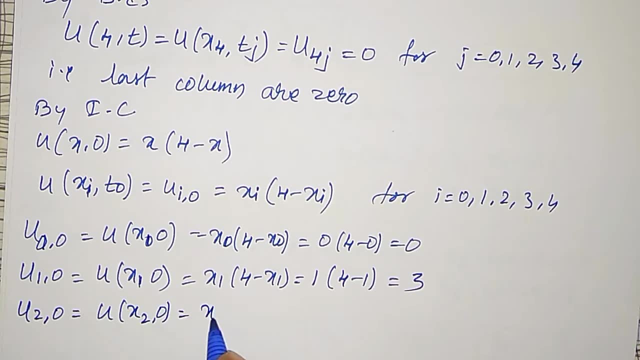 1 into 4 minus 1, which is equal to 3. I am going to get like that, U of 2 comma 0, U of x 2 comma 0, my x 2 into 4 minus x 2, that is, 2 into 4 minus 2. 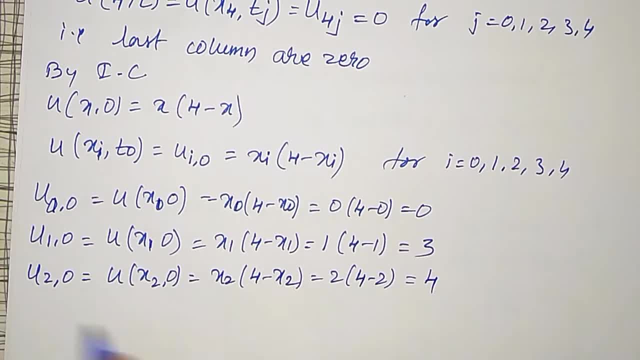 2. 4 minus 2 is 2. 2 into 2 is 4. like that U of 3 comma 0 equal to U of x 3 comma 0, that is, x 3 into 4 minus 2, 4 minus x 3. 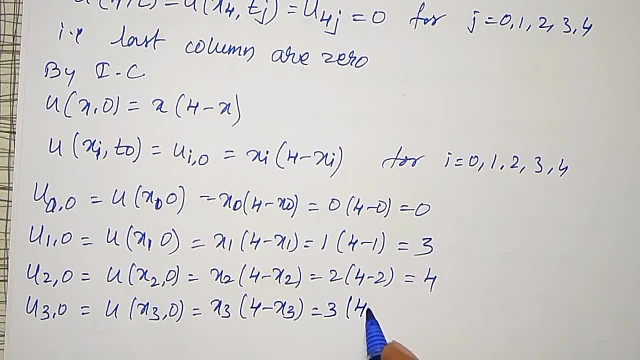 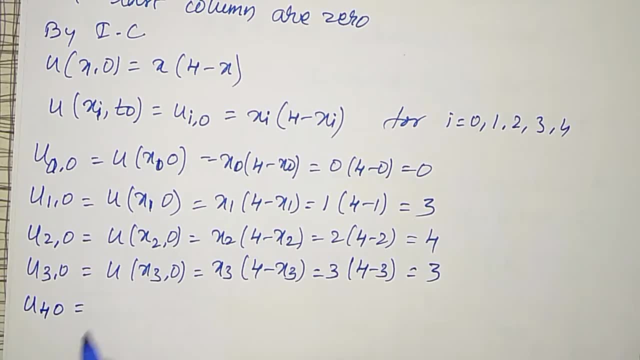 that is x, 3. value is 3. 3 into 4 minus 3. 4 minus 3 is 1. 1 into 3 is 3. like that, U of 4 comma 0, you can find out that is U of x, 4 comma 0. 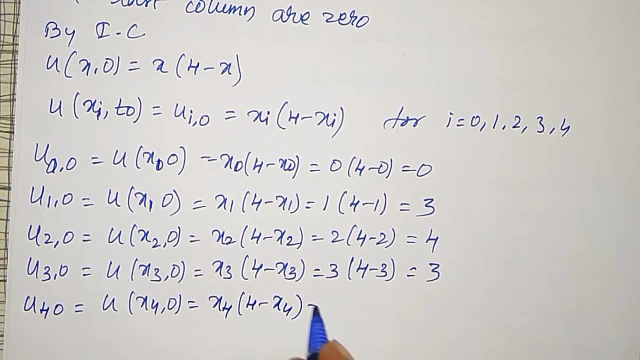 that is x 4 into 4 minus x 4. that is 4 into 4 minus 4. but 4 minus 4 is 0. 0 into 4 is again 0. using these values in the table, what I am going to get? 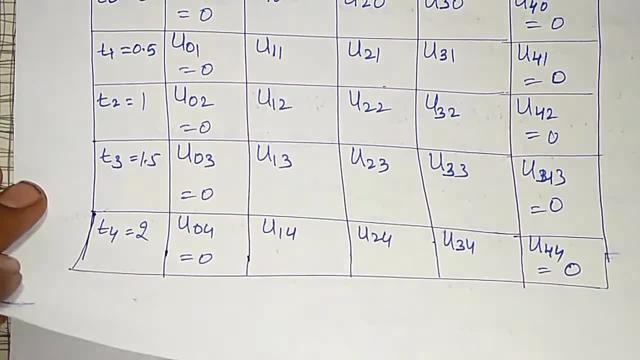 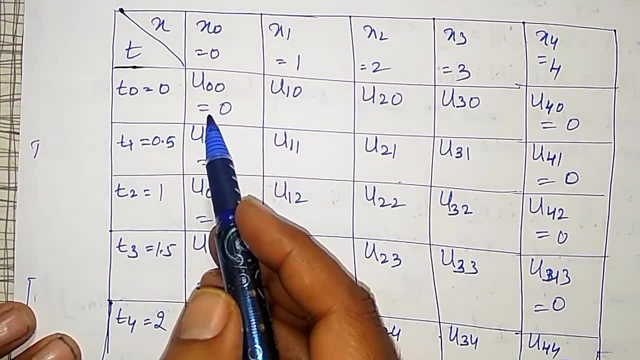 that is in the table. if I am going to use them, then what happens here? let us just find out: U of 0 comma 0, equal to 0. U of 0 comma 0, equal to already 0. is there next? U of 1 comma 0, equal to 3. 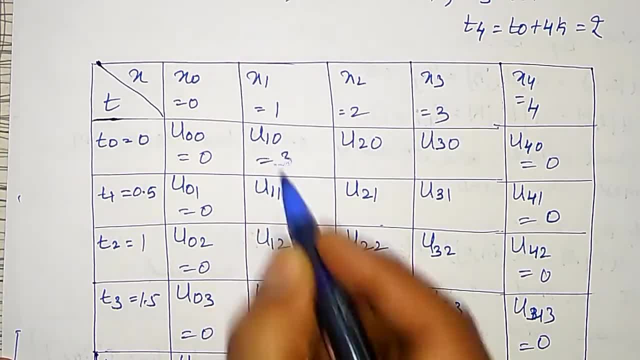 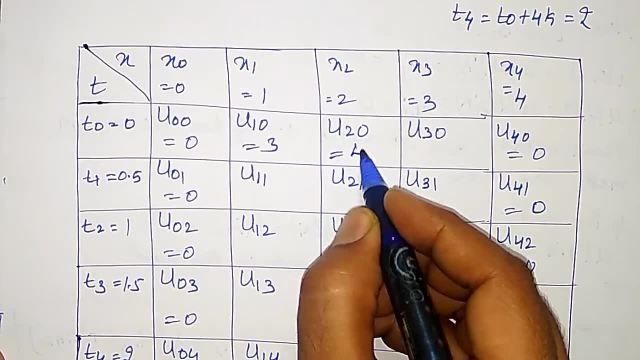 U of 1 comma 0, that I will equal to 3. I will substitute like that: U of 2 comma 0, equal to 4. U of 2 comma 0, equal to 4. next, U of 3 comma 0, equal to 3. 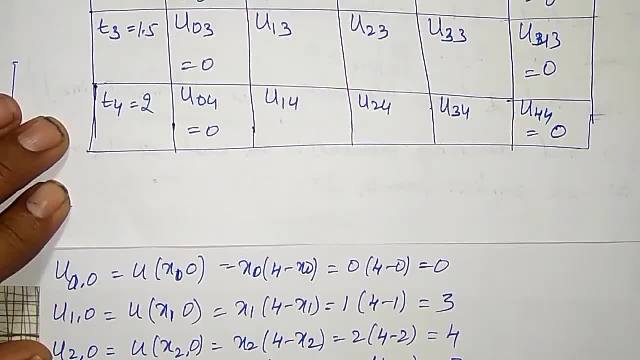 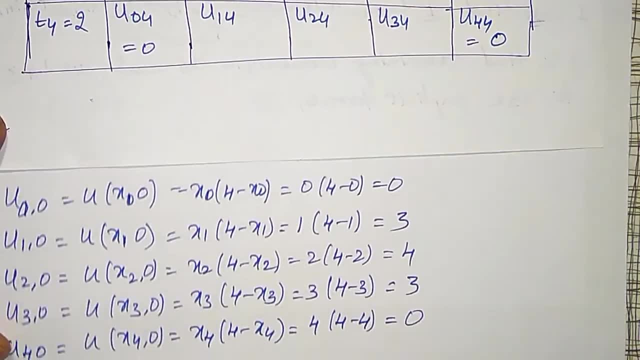 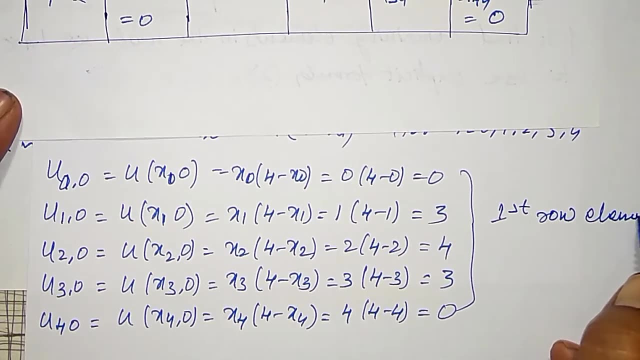 U of 3 comma 0 equal to 3 and U of 4 comma 0 equal to 0, and already it is there from the boundary conditions. therefore, using this initial condition, I have calculated the first row elements. first row elements. ok, then to find the second row elements. 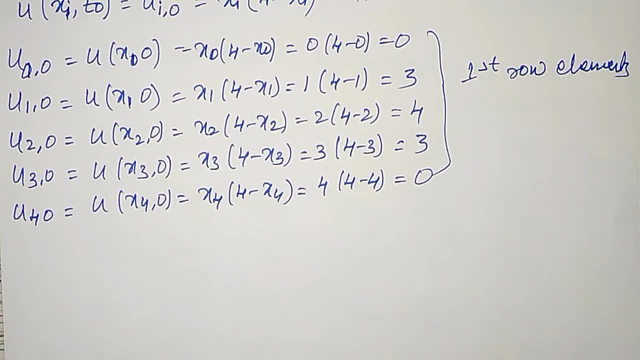 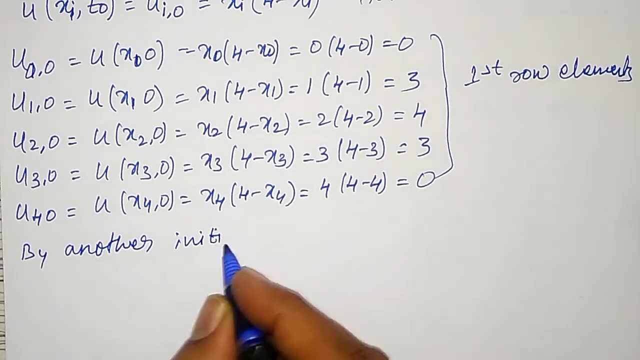 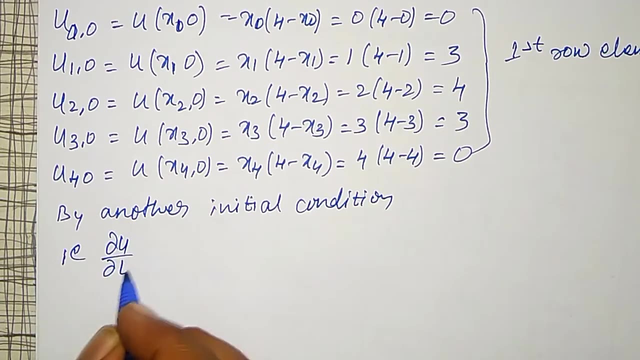 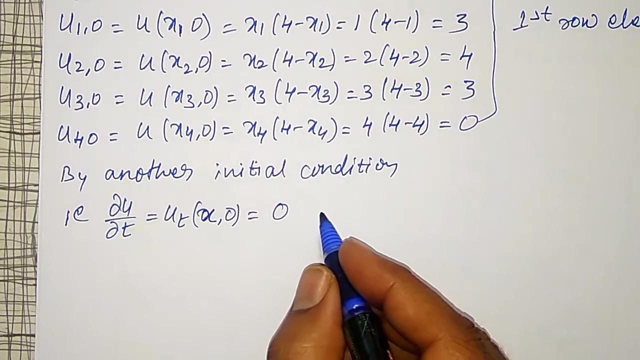 second row elements. let me use another initial condition by another initial condition. initial condition that is dou U by dou t, that is U t at 0 comma. sorry, x comma 0 is equal to 0, but using this in explicit derivation, I derived the formula that: 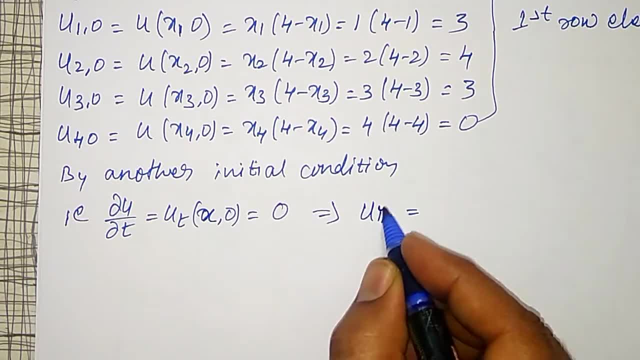 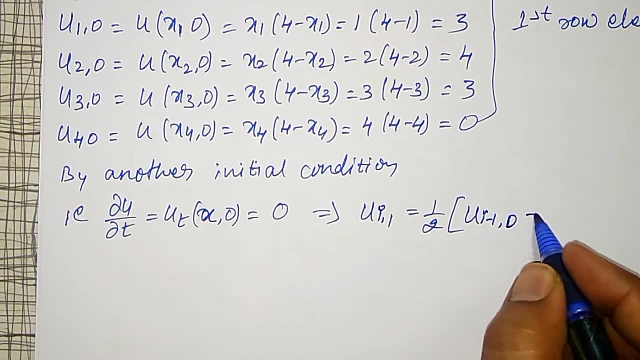 which implies U i comma 1 is equal to 1 by 2 times 1 by 2 times U i minus 1 comma 1, 0 plus U i plus 1 comma 0, for i equal to 0, 1, 2, 3 and 4. 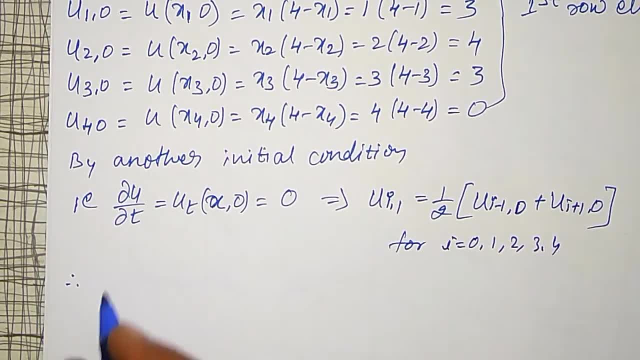 ok, therefore, therefore, U 0 comma 1, equal to 1 by 2 times I am using: i equal to 0, therefore, minus 1, that does not exist. therefore, i equal to 0 will not exist. therefore, let me start with 1: 1. 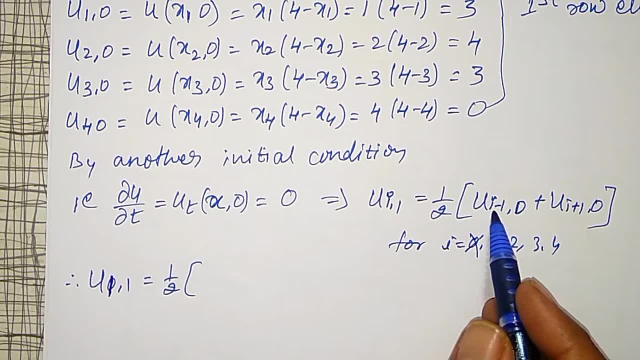 for i equal to 1, 1 i equal to 1, it will become U 0, 0 plus U. i plus 1, i equal to 0. therefore, it is sorry, i equal to 1, 1 plus 1. U 2 comma 0. 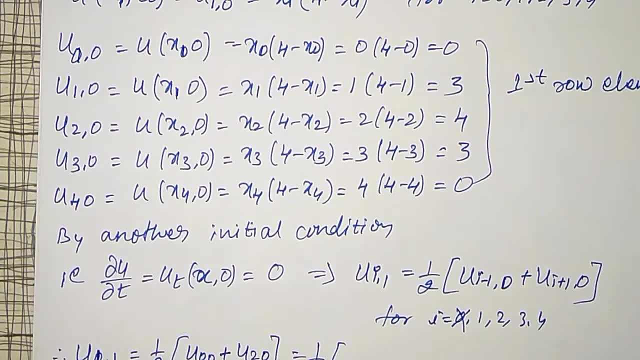 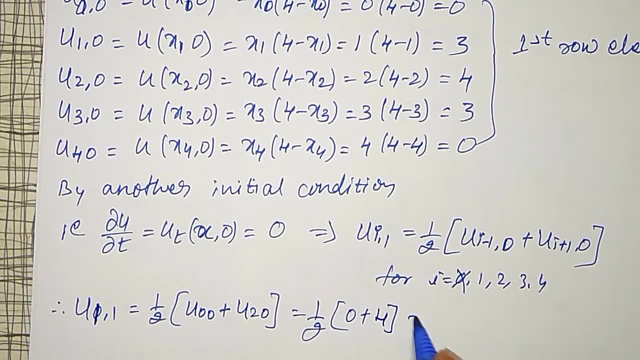 and these two already have calculated U 0, 0 and U 2, 0. its values are 0 and 4, therefore 0 plus 4, 0 plus 4 is 4, 4 divided by 2 is 2, like that, like that. 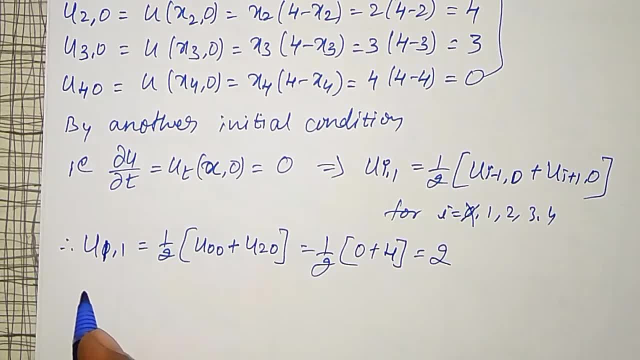 i equal to 2. if I am using U 2, 1 equal to 1, by 2 times i equal to 2. I am using 2 minus 1, that is 1 comma 0 plus i equal to 2. 3- U 3 comma 0. 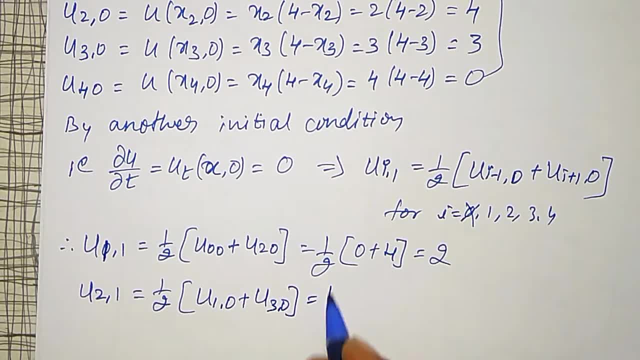 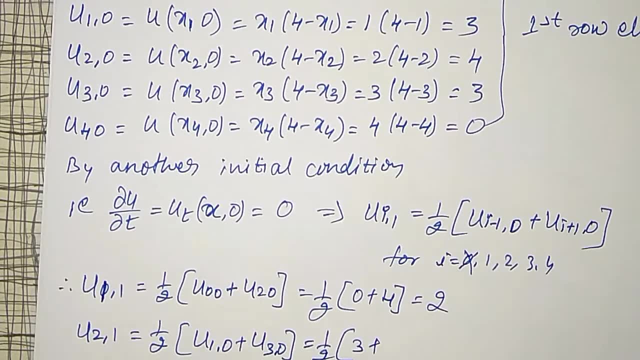 1 by 2 times U 1: 0. already I have calculated that is 3 plus U 3 comma: 0: 1 by 2 times U 1, 0, 3 0, 3, 0. also calculated, that is also 3. 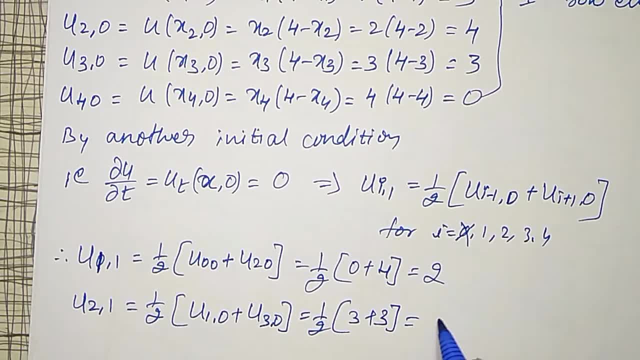 3 plus 3 is 6. 6 divided by 2 is again 3. like that, i equal to 3. I can use U 3: 1 equal to U 3. 1 equal to 1 by 2 times U 3 minus 1. 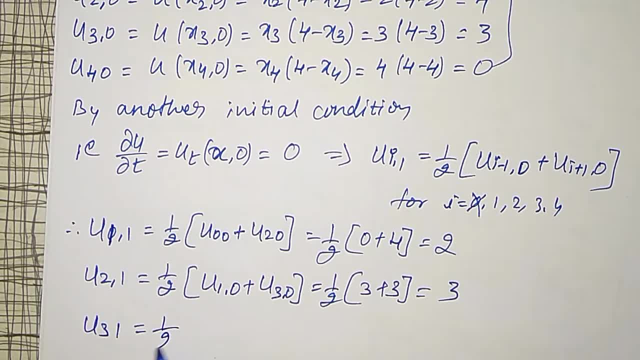 2, 2 comma 0 plus U i plus 1 i is equal to 3, 4 comma 0. 1 by 2 times U 2, 0, 1 by 2 times U 3 minus 1 2 2 comma 0. 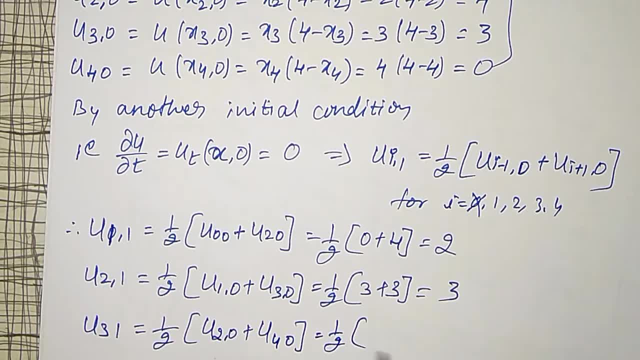 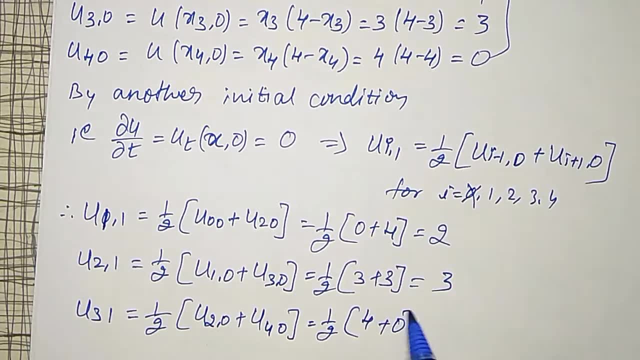 plus U, i plus 1, i is equal to 3, 4 comma: 0: U 2, 0 is already 4. is there? 4 plus U: 4: 0 is a 0, which is equal to 2. if you are using i, equal to 4. 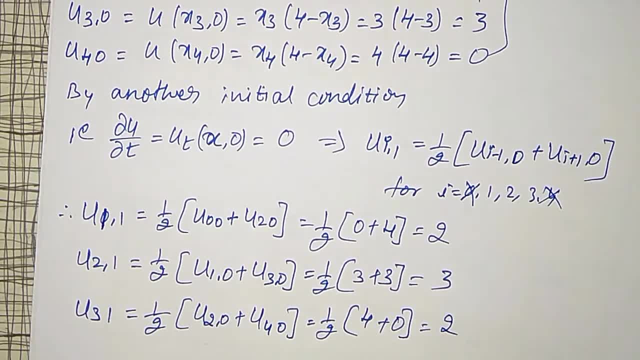 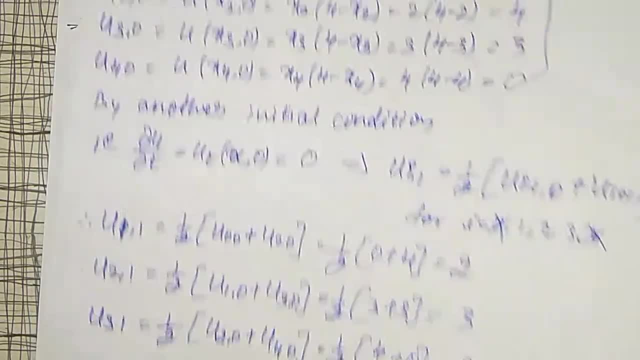 then it will become 5, but it does not exist. therefore, for 1, 2, 3, only substituting these: U 1, 1, U 2 1, U 2, 3, 1 in the table. those values are nothing but ok, these values. 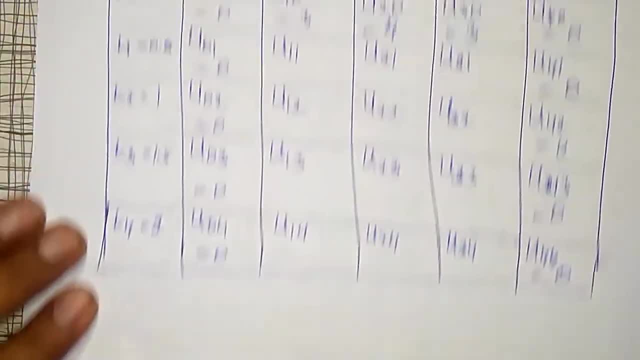 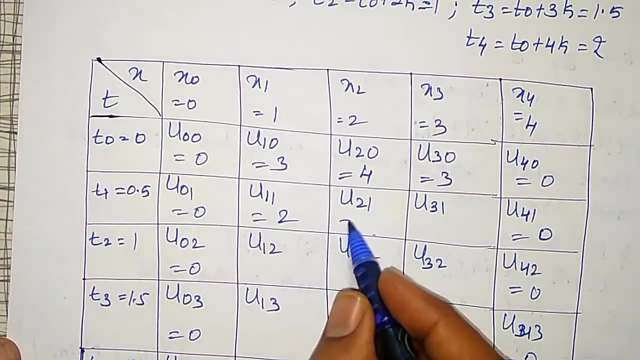 that is what I can. U 1: 1 equal to 2. U 1: 1 is here, U 1: 1 is 2, like that, U 2: 1 is 3. U 2: 1 is 3, then U 3: 1. 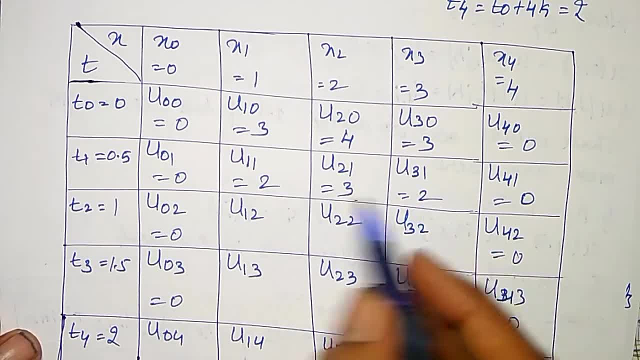 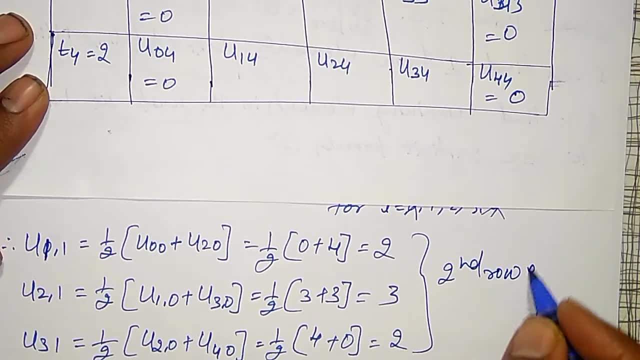 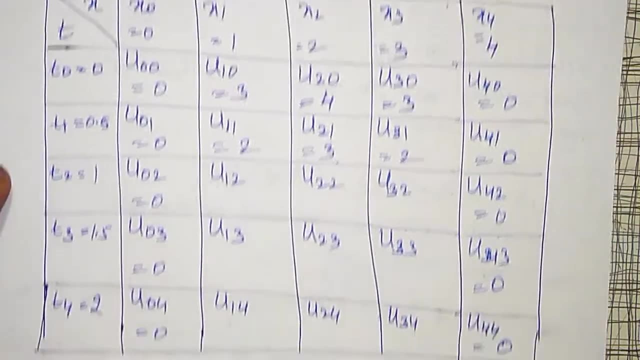 is equal to 2, correct? that is equal to U 3, 1 equal to 2. this is nothing but second row elements. I have calculated. these are nothing but second row elements. ok, therefore, using all 4 conditions, I have calculated 2 columns and 2 rows. 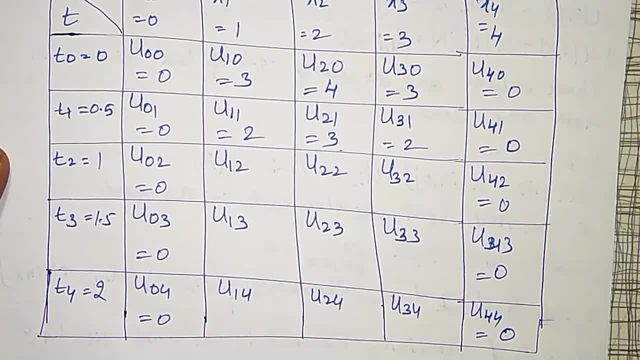 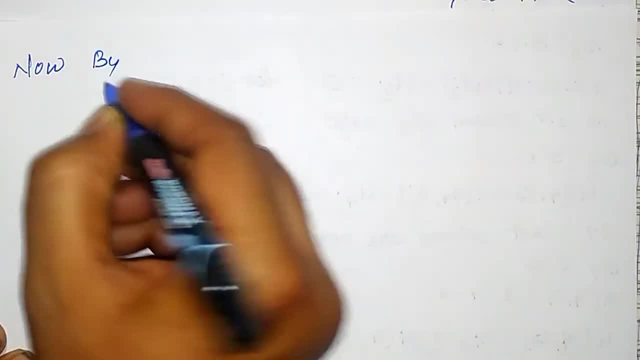 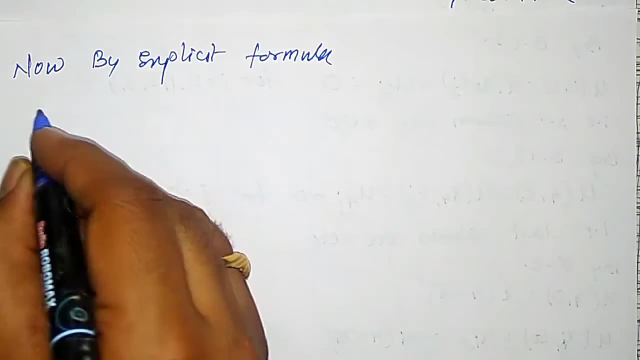 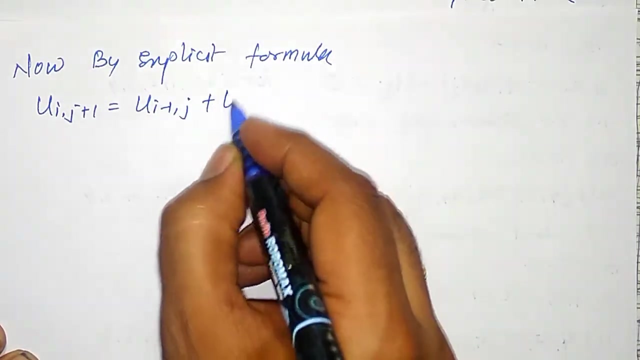 then to find out these remaining 9 elements, I will use the explicit formula now. I will come back here now by explicit formula. explicit formula, that is: U i comma j plus 1 is equal to U i minus 1 comma j plus minus U i comma. 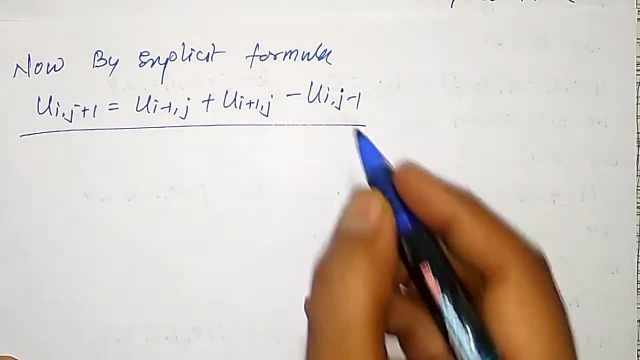 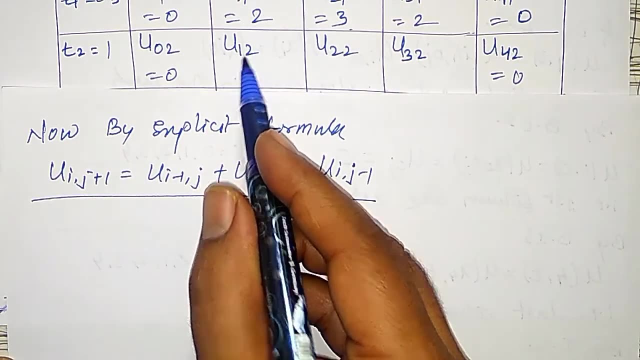 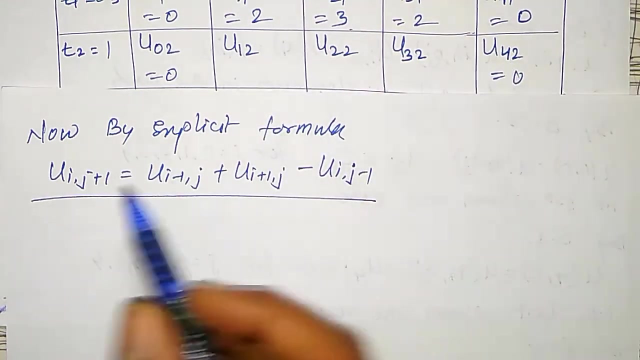 j minus 1. I am having formula, therefore, to find out this in the table. in the table I want to calculate what here: U 1, 2. now, therefore, i equal to 1 and j equal to 2, j equal to 2, 2 is. 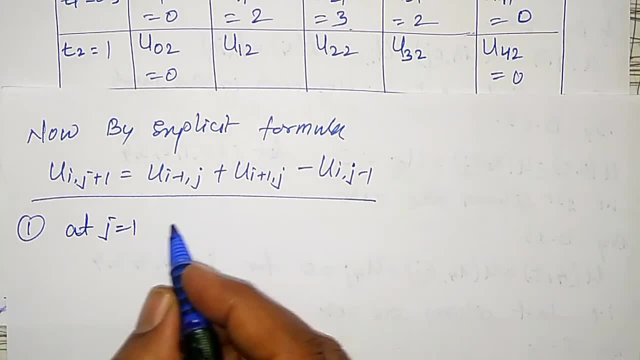 remained ok, therefore, to get: and for i equal to 1, 2, 3, that is, let me use: j equal to 1 and i equal to 1, i equal to 1, U 1 comma 2 equal to ok, U 1, 2 equal to. 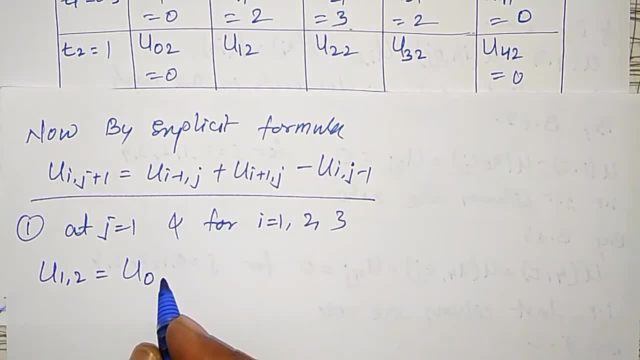 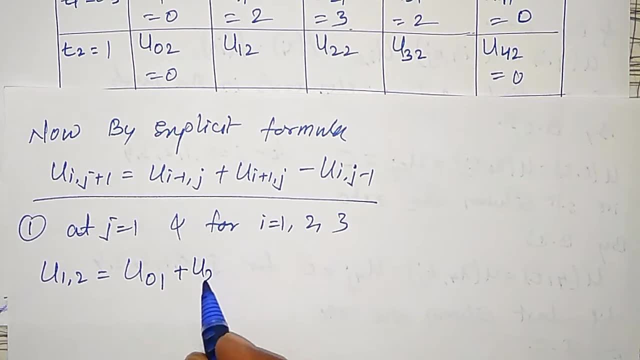 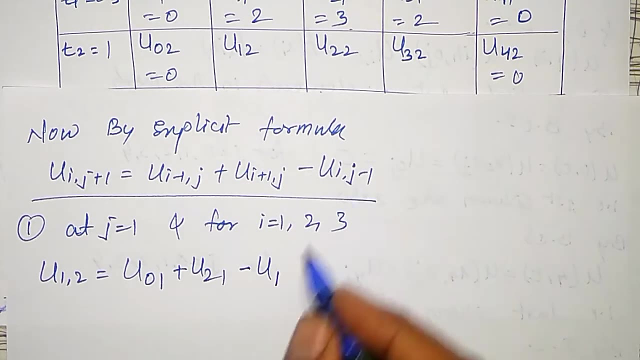 U i equal to 1. I am using therefore U 0 and it is j equal to 1, plus U i equal to 1 and j equal to. i equal to 1 means i equal to 1, 1 and j equal to 1. 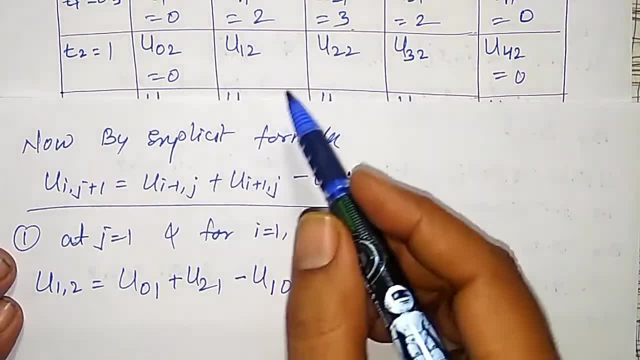 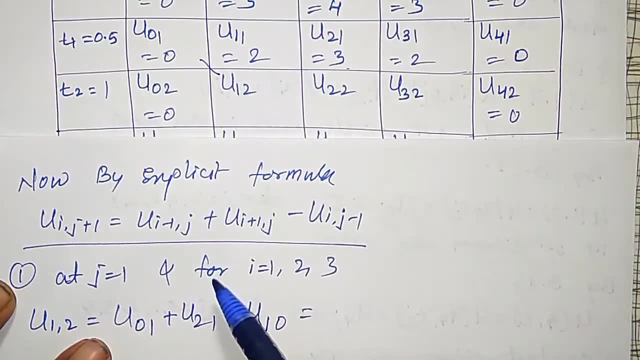 0 already. these values I have been calculated here to find out U 1- 2. U 0- 1- this value ok- and U 2- 1- this value, diagonal value that is, I will use here- 0 plus. this value is 3 minus. 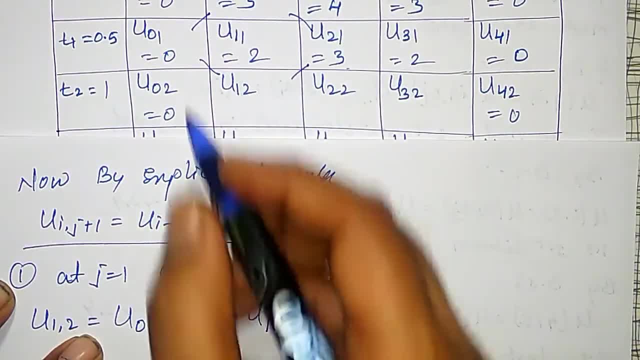 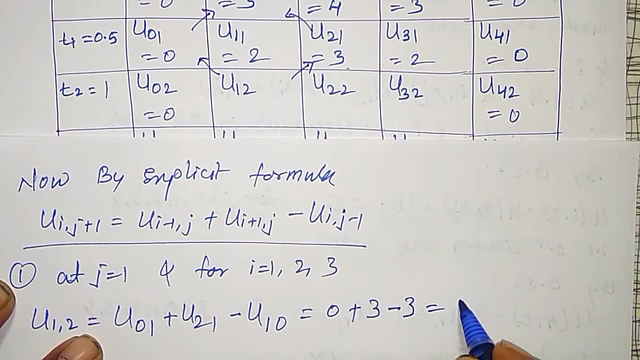 U 1: 0, the diagonal of this, this diagonal first, and then diagonal of these two, will come 3. ok, that is 3. I am going to get it as equal to 0. therefore, U 1: 2 is equal to 0. similarly for: 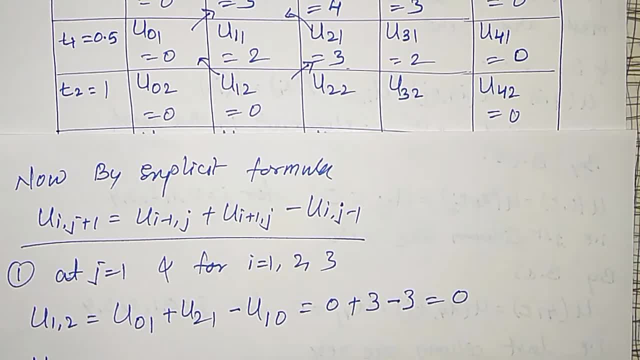 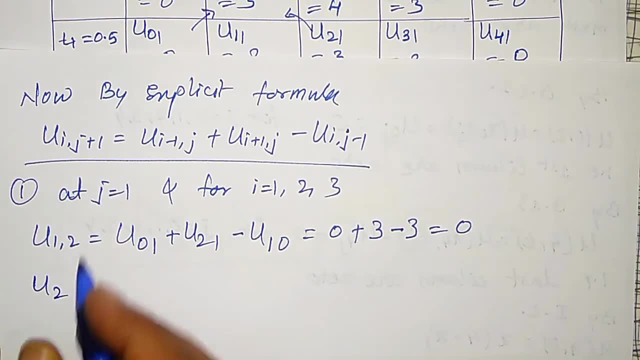 j equal to 1 and i equal to 2. now U ok. next, j equal to 1, i equal to 2. therefore, 2, 2 equal to 2, 2, that is U 2, 2. to find out this, U 2, 2. 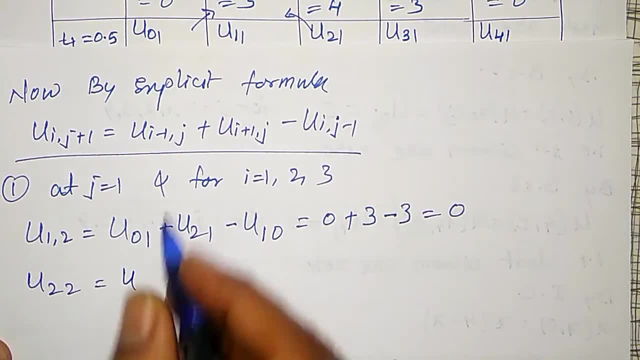 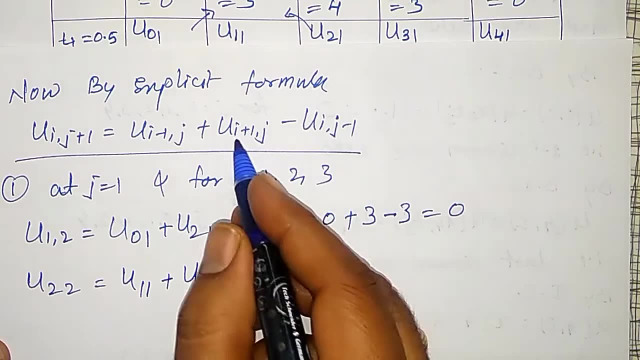 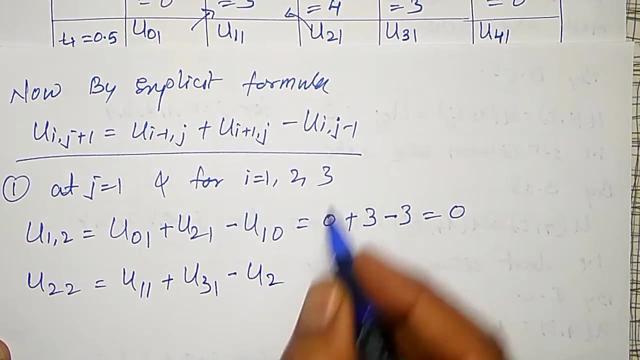 this becomes U of i equal to 2, 2 minus 1. is 1. j equal to 1 plus U i equal to 2. 2 plus 1. 3 j equal to 1 U 3. 1 minus U of j i. 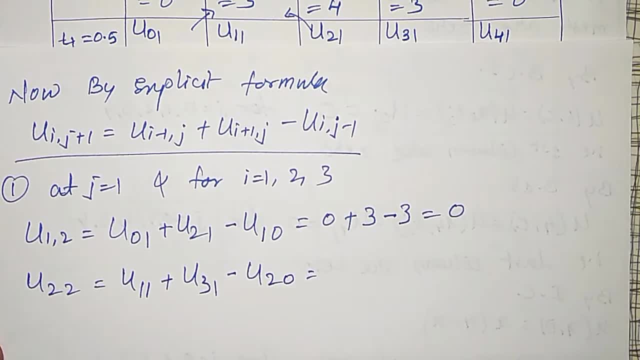 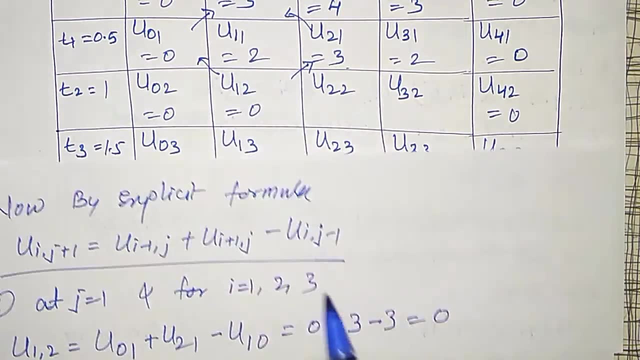 i equal to 2, 2 and j minus 1. again it is 0. and from the table you can just go through this: U 2, 2, its diagonal element. U 1- 1 element, it is 2, ok, and U 2, 2. 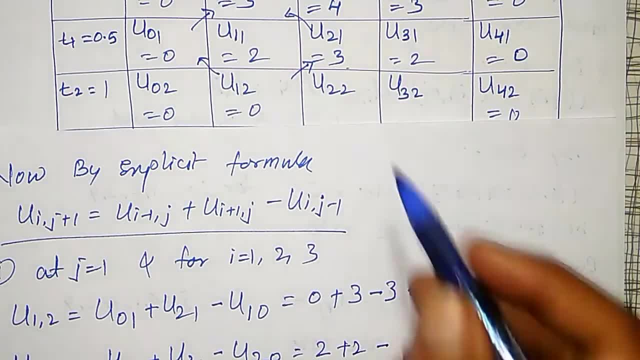 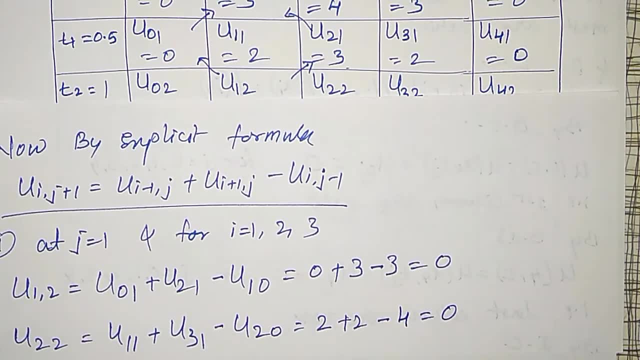 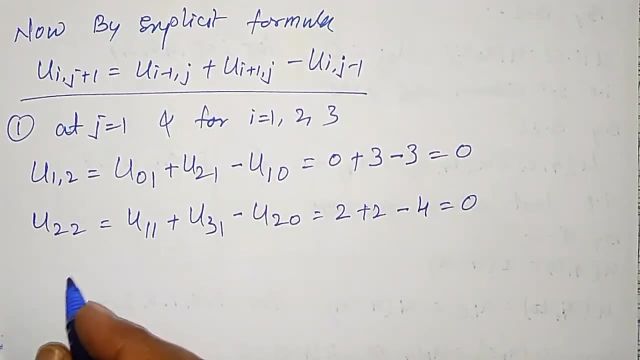 again, U 3- 1 is 2 plus 2 minus these diagonal elements is 4, which is also equal to 0. ok, therefore, this also equal to 0. next, to find out U 3- 2. to find out U 3- 2. 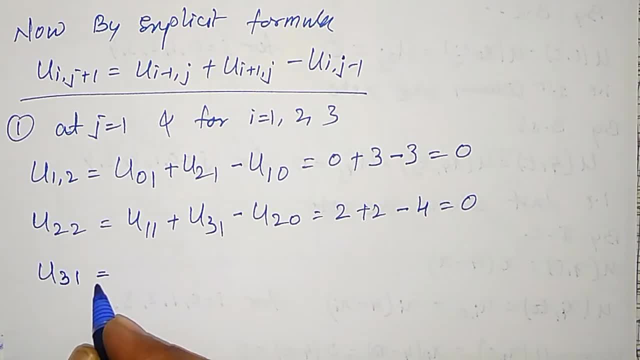 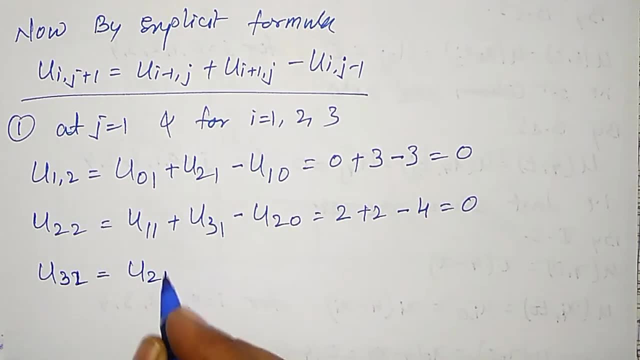 i will use U 2- 1, that is U 3, 1 equal to sorry, U. 3. 2 equal to i equal to 3. 3 means 3 minus 1, 2 and j equal to 1 plus U i, equal to. 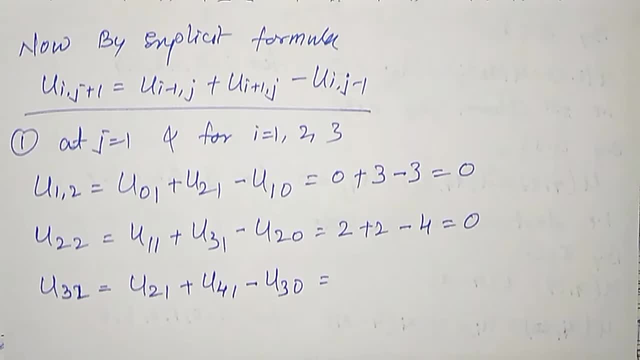 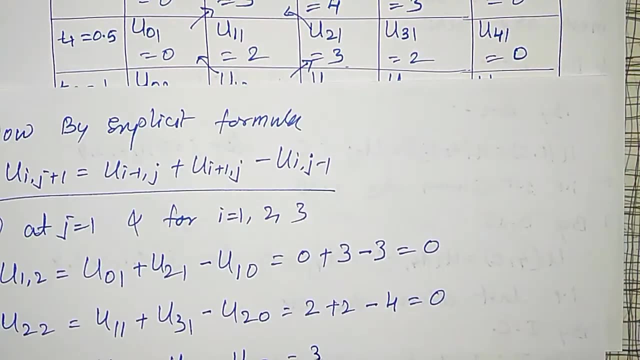 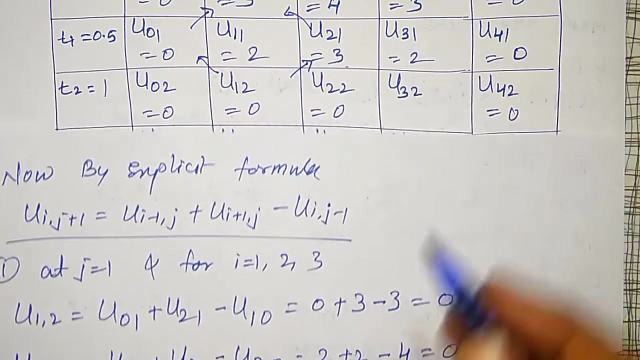 3, 3 plus 1, 4 and j equal to 1 minus U of 3 comma 0. from the table you can just check out U 2 1, U 3- 2 to find out U 2 1 minus U 3 0. 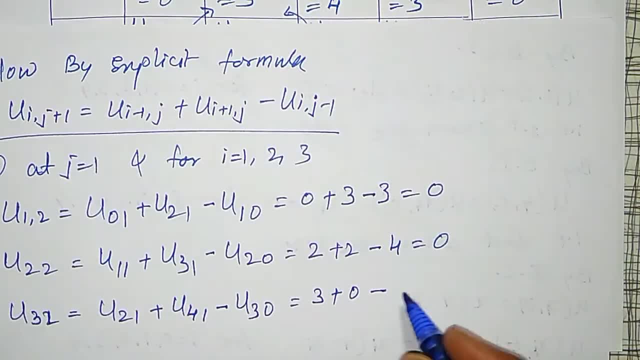 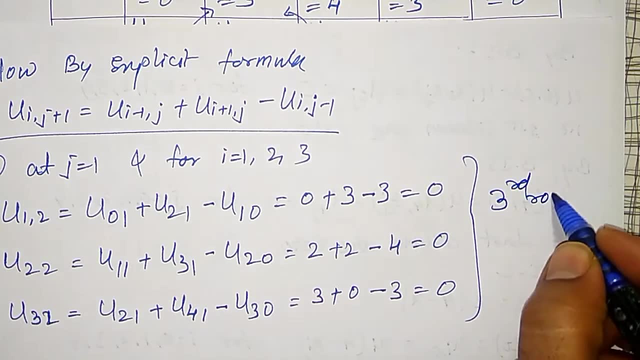 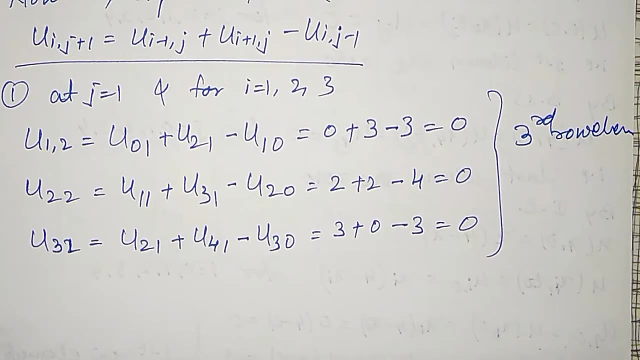 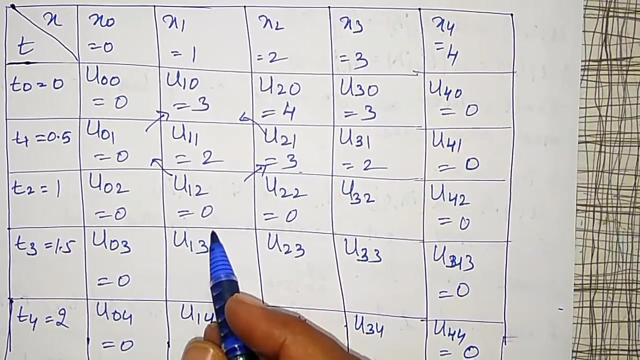 U 3, 0, U 3, 0 is 3. therefore, 3 minus 3 is again 0. this will give you the third row elements. third row elements: ok, like this. ok, this mesh value, this one, whatever i have calculated, just you can check here. 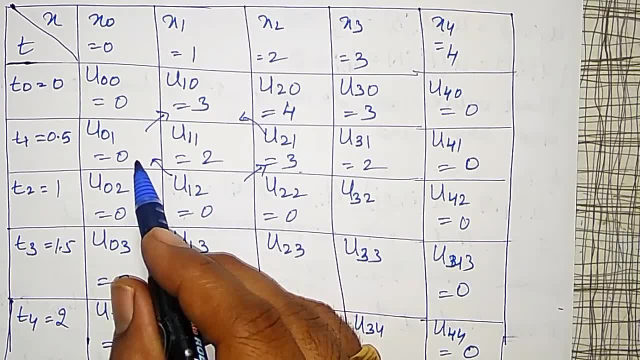 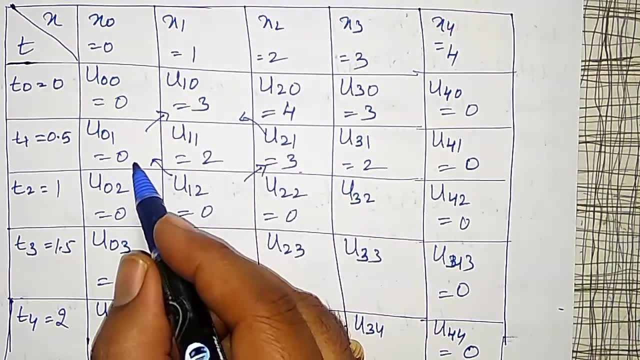 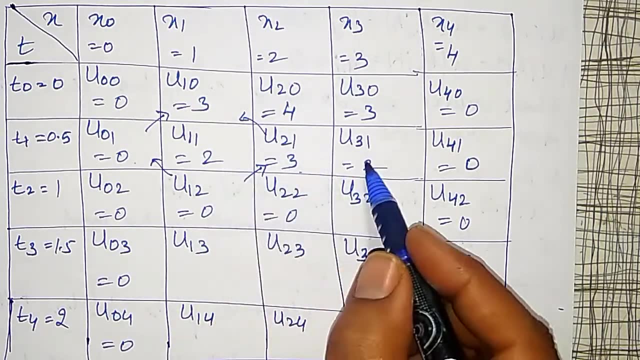 explicit formula to find out U: 3, 2 diagonal of this diagonal of this, both sides, upper diagonals and diagonals of this one, calculated minus that 0 plus 3 minus 3, therefore it is 0. like that to find out this 2, 2 element. 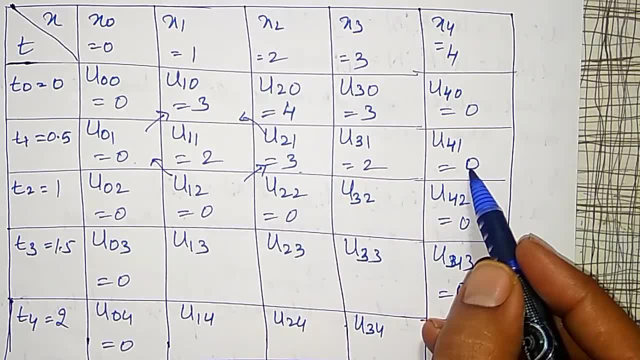 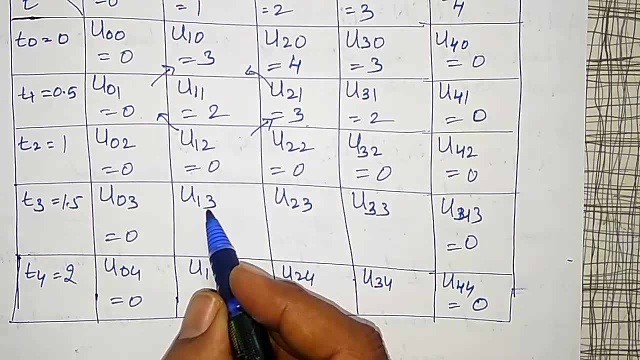 diagonal 2 plus 2 minus 4. i have done to find out U 3, 2, 3 plus 0 minus 3, equal to 0 like that, without using explicit formula. in substitution we can use diagonal element: 0 plus 0 minus 2. 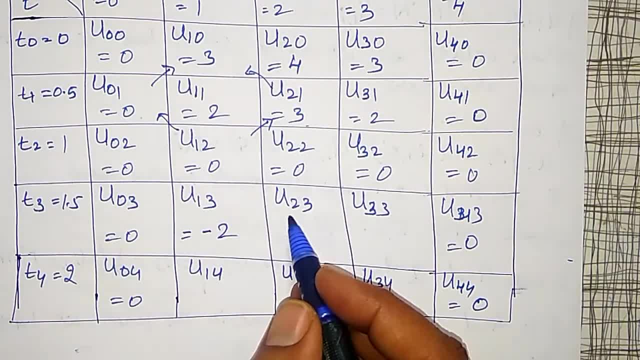 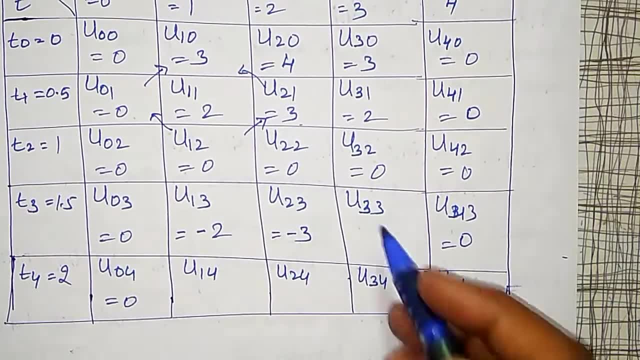 therefore, which is equal to minus 2. i am getting like that: U 2, 3, 0 plus 0 minus 3 minus 3. i am getting to find out: U 3, 3, diagonal element 0. this diagonal element 0 minus 2.